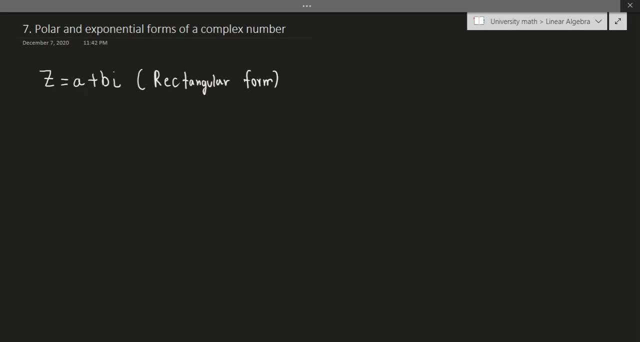 complex numbers a lot more easily and whatnot. But this isn't always the best kind of situation to work with, As before when we did, for example, when we did complex arithmetic, in order to divide complex numbers, say a plus bi, divided by c plus di, we first had to multiply. 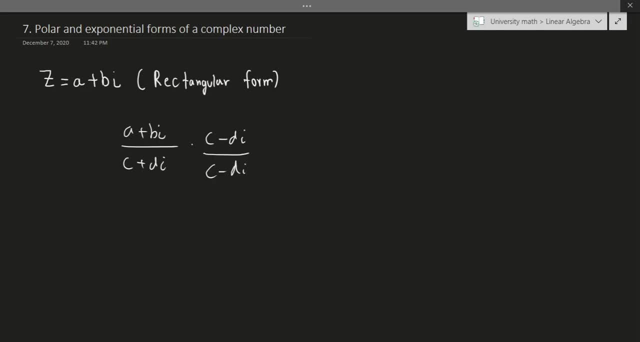 by the complex conjugate On top and bottom in order to do any kind of arithmetic. That's not very convenient because it takes a very long time to work on this. So is there an easy way to kind of write out complex numbers in order to make our life a little bit easier? Yes, there is. So one way to kind of write. 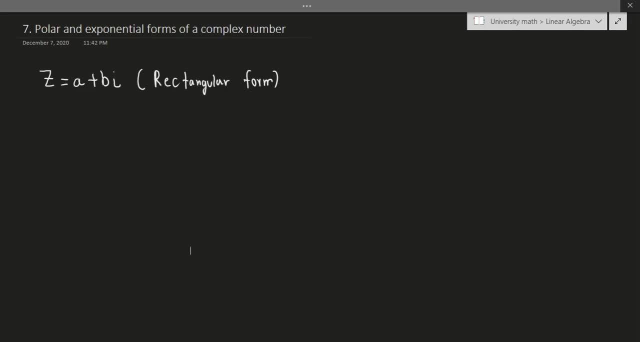 a complex number in a different way is use something called the polar form. So what is the polar form of a complex number? So let's go ahead and talk about that instead. So let me just move this over. Okay, so now let's go ahead and plot a complex number. So we call that a complex. 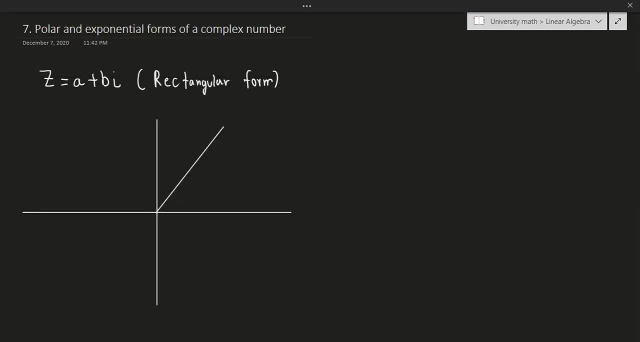 number is essentially just, can essentially just be plotted on the coordinate system. So there we go, And there we go. So this complex number, right there is the complex number z equals a plus bi. So this x coordinate, right there, that's a. this x coordinate, or this coordinate, right there, that's b. And we can, we know that this is the. 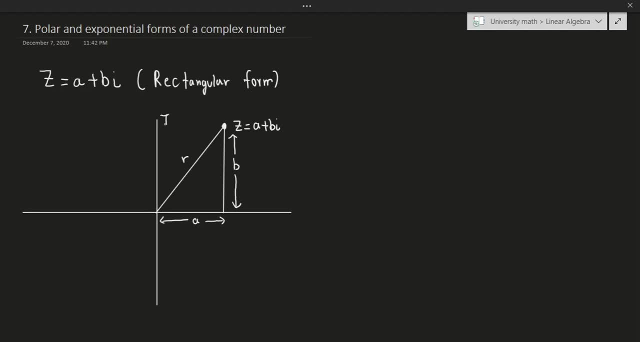 hypotenuse, which I would call r. So just be very clear: this is the imaginary axis and this is the real axis. Okay, now here's the thing: Because this is a triangle, I can define an angle, theta, right there, And the angle of this thing can be measured using the tangent ratio. So we can use tan. 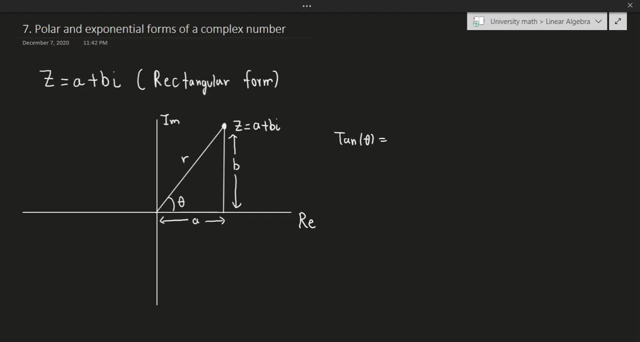 theta equals b over a and use that to find the angle. So that's certainly one way. So we'll- we'll come back to it a bit later, But the point is I can use the angles to kind of relate this. So now, 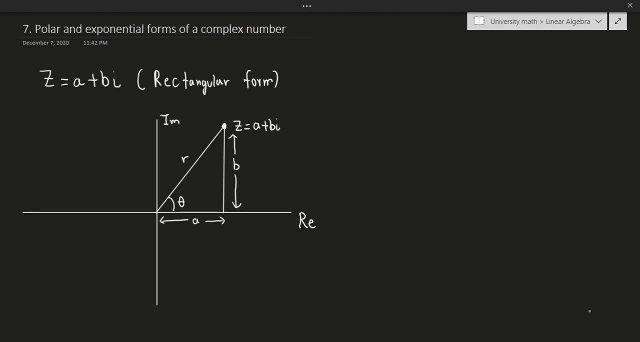 let's talk about what polar form is. Polar form is essentially using something called polar coordinates to measure complex numbers, using angles and trigonometric ratios instead of Cartesian coordinates. Instead of a plus bi, I've used angles and trigonometric ratios to kind of measure this. So how does that? 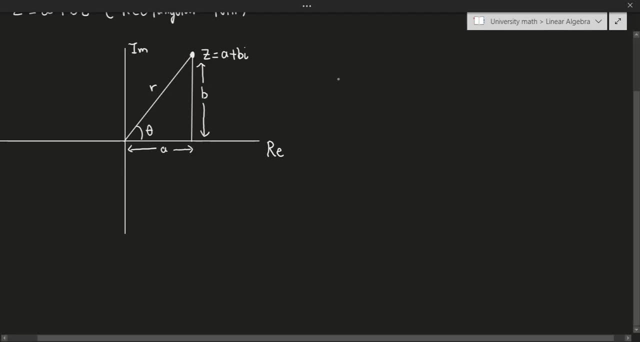 work exactly. So let's just kind of define the Cartesian polar coordinate system, really very briefly. This will be covered a little bit later in calculus two in a lot more detail, But let me just give a brief overview. So let's define a few trigonometric ratios. So let's define a few. 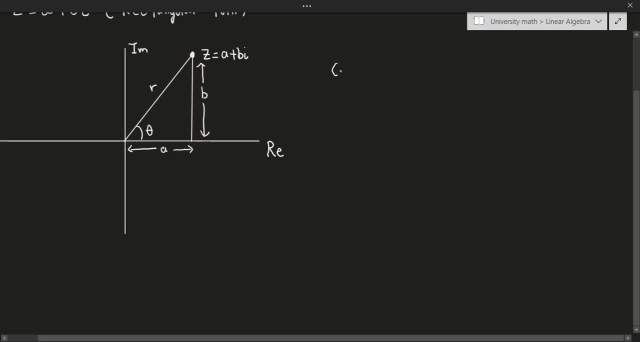 trigonometric ratios. So we know for a fact that the cosine of theta is equal to the adjacent toward hypotenuse. So in this case that'd be a over r. Here we know that sine of theta is equal to opposite over hypotenuse, that's b over r. So that means by definition, 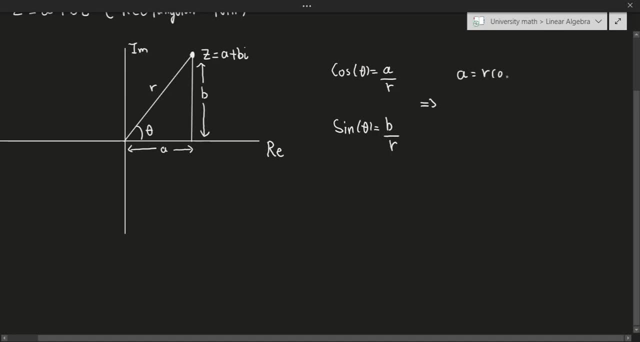 we get the following: we get a equals r cosine of theta, And we also get that b equals r times the cosine of theta. Okay, so we get two ways to relate A and B: using the radius or not radius, the hypotenuse and the angles, instead of using Cartesian coordinates. So how else can we kind? 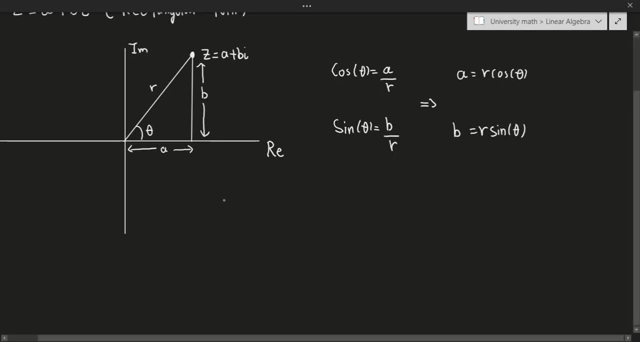 of relate these two things together. Well, let's try the following. Let's see what happens when we go a squared plus b squared. Well, a squared plus b squared is, by definition, it's going to be cosine of theta, all squares. it's going to be r squared, cosine squared, theta plus r squared. 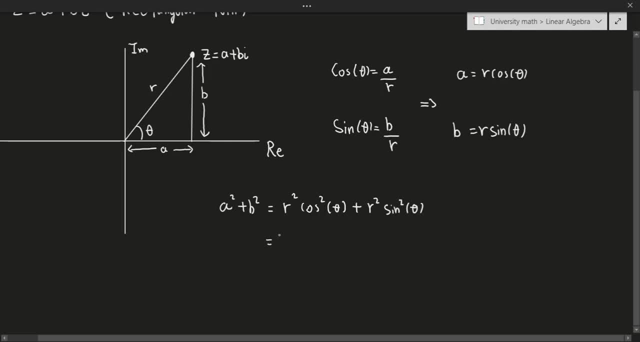 sine squared of theta. And then, when I factor the r squared out, we get cosine squared of theta plus sine squared of theta. Okay, but that's just one, because that's a very, that's a fundamental trigonometric identity. So we obtain the following: that a squared plus b squared is equal to r. 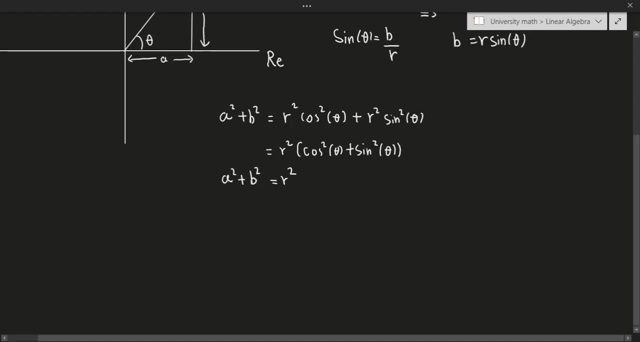 times the radius of theta plus r squared, that is the radius. it's also square root of a squared times the radius of theta plus r squared times the radius of theta plus r squared times the radius of theta. And that's what we're going to say. So, in other words, we can define the complex number. 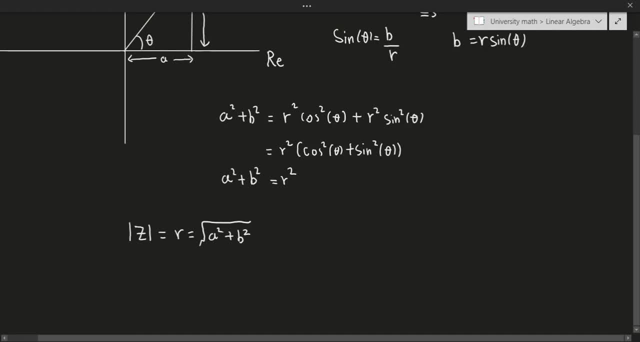 in the following way: we can say that the modulus, or the absolute value of the complex number is r, which is equal to the square root of A squared plus B squared. So so, in other words, the length for the argument. so let's go ahead and write that down. so let's just go b over a. well, b over a would be r. 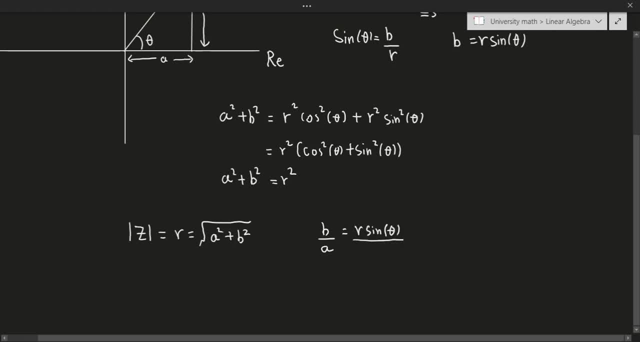 sine theta divided by r cosine of theta, but then the r's cancel and then sine theta over cos. theta by definition is the tan of theta. so by definition we get the following situation: we get b over a equals the tangent of theta. so by definition we get theta equals inverse tan of b over a. 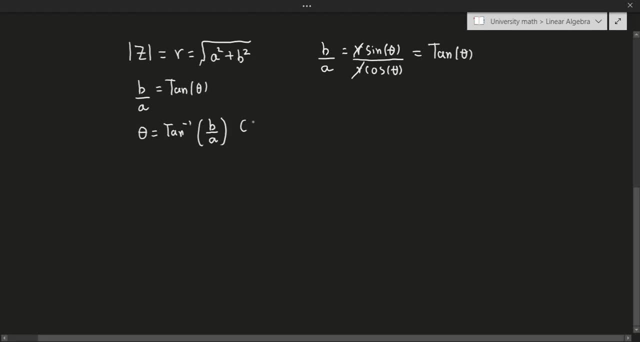 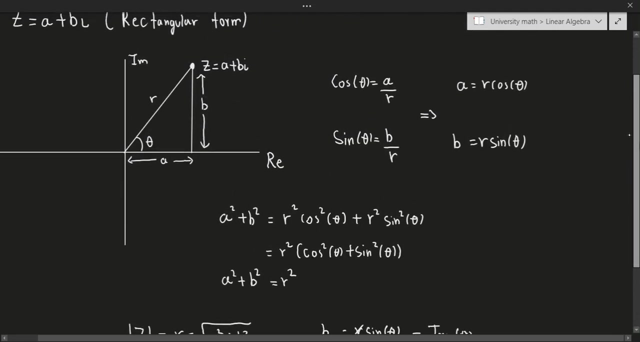 okay, so this right here is called the argument. okay, so this is very interesting. so because of that, we can now kind of evaluate this in the following way. so instead of using cartesian coordinates, we know that the tangent of theta is the tangent of b over a, so we can now kind of evaluate this. 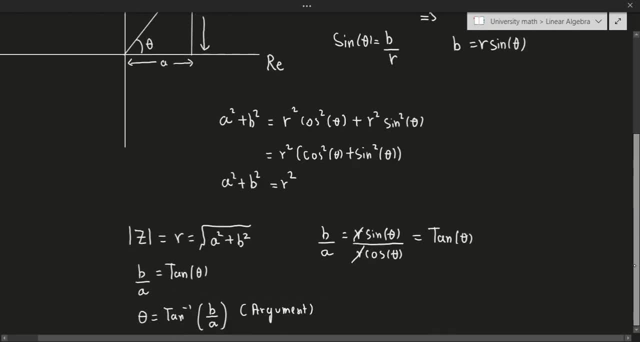 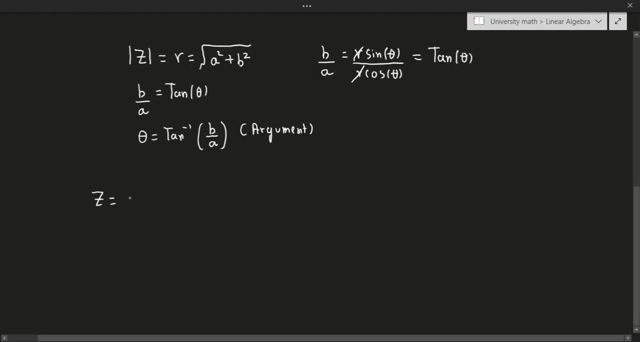 we know what a and b are now, so we can go ahead and replace a and b with the trigonometric variance. so as a result, if z equals a plus b i, we can replace a with r cos theta and then b with r sine theta times i, and then we can factor the r out, so we get r cosine of theta plus. 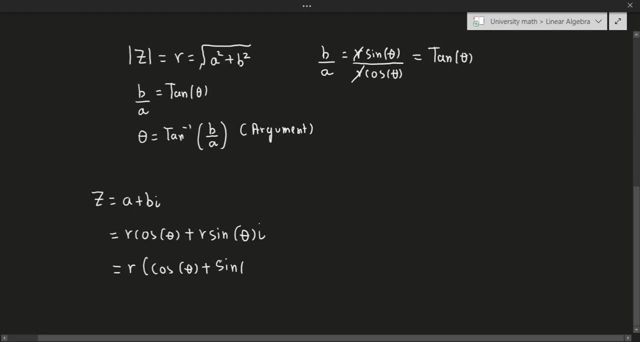 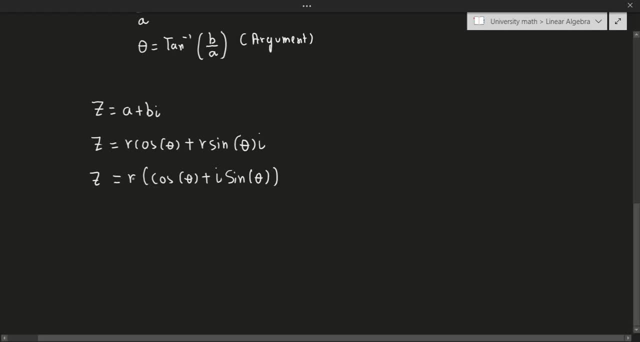 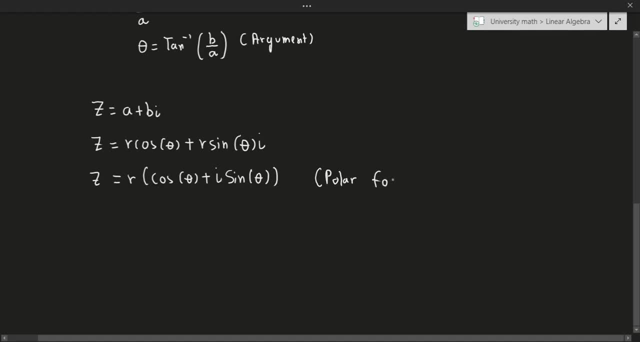 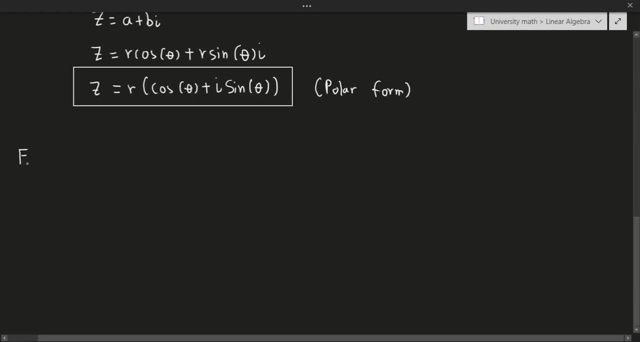 now, that being said, let's do two examples based on this rectangular form, and then we'll talk about a more important thing called the exponential form. so the first example is the following: so write: z equals minus 1 plus root, 3 times i in polar form. 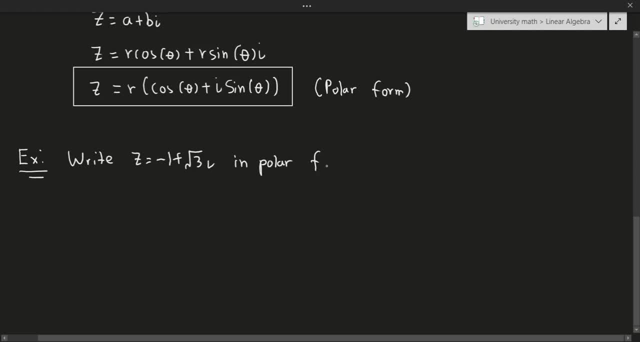 okay, so how do we do this? well, we can do the following. so we have to. so remember that for polar form, we have r times cosine of theta plus i. okay, so we need to calculate r is in order to approach this times sine of theta好, so we need to calculate r is and we need to calculate what theta is in order to approach this. so r is. 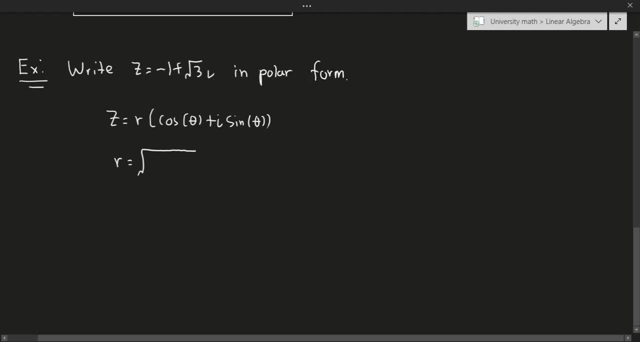 equal to the square root of a square plus b squared, so it's minus one squared, plus root three, uh squared. so let me just fix that a little bit. so this gives us r e plus v nr of equals root three, square, that's three. minus one square, that's one. So we get the square root of. 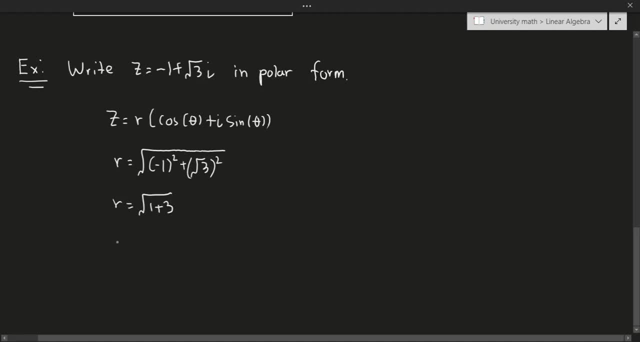 one plus three. but one plus three is four. So we end up getting the square root of four, which is, by definition, just equal to two. Okay, the next thing we need is the angle. So we do that using the argument. So the argument is tan of theta is equal to b over a. 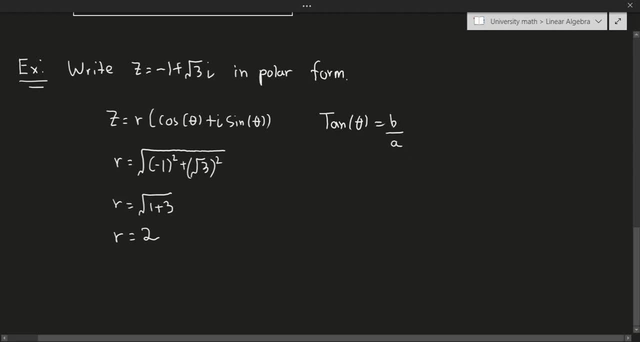 Okay, so that's fine. So let's go ahead and calculate this. So we get: tan of theta is equal to root three divided by minus one. So theta is equal to tan inverse of minus root three. And if you use a unit circle or your triangles to do this, or a calculator, you can go ahead and 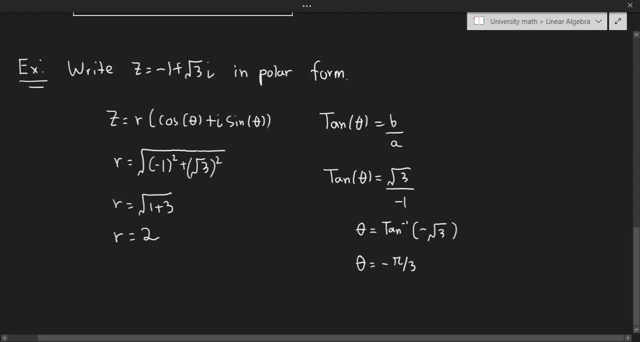 get minus pi, root three when you do this. So we get. tan of theta is equal to b over a, So we get. but here's the problem. Let's go ahead and plot the complex number for a second, So just to give you a sense of what's going on. This complex number is minus one and root three. 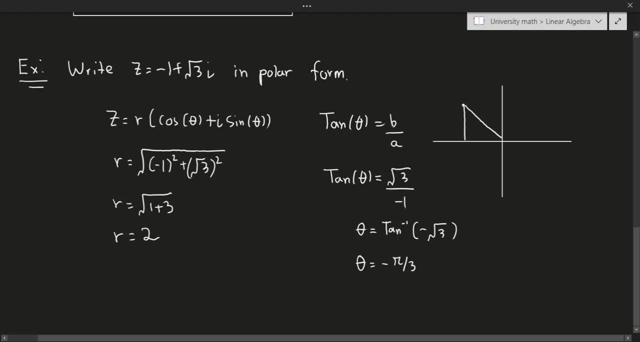 That's here roughly speaking. But the problem is that minus one is so minus one x, and then root three is the y value And this gives us two. That's fine, But the problem is that this angle minus pi over three is an angle, So we get tan of theta is equal to b over a, So we get tan of theta. 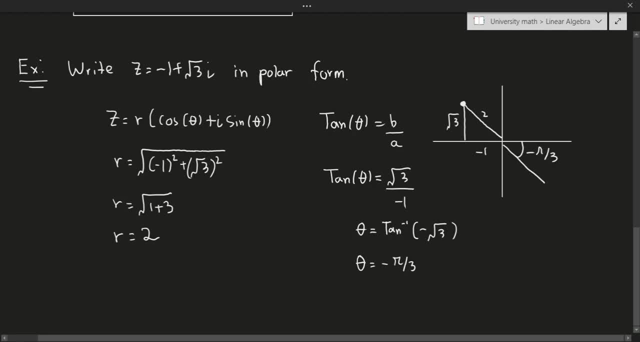 in this quadrant, right there. That's a bad thing, because we need to make sure that the angle that we get is in this quadrant. Well, according to the cast rule, so there's only two places where the tangent is negative: here and here. So in order to get to this quadrant, we can just add: 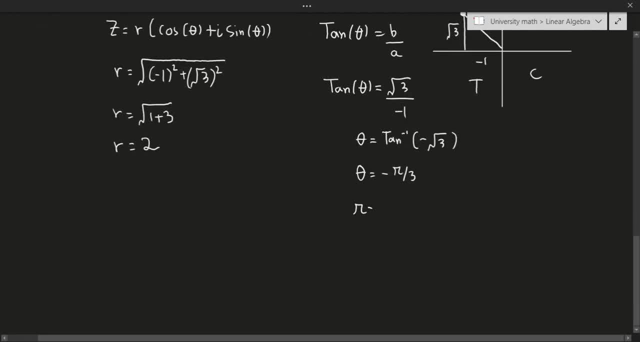 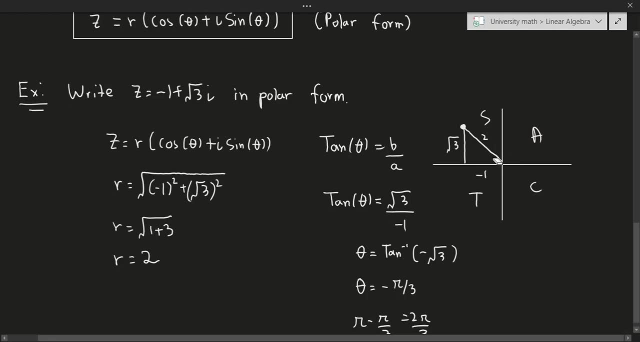 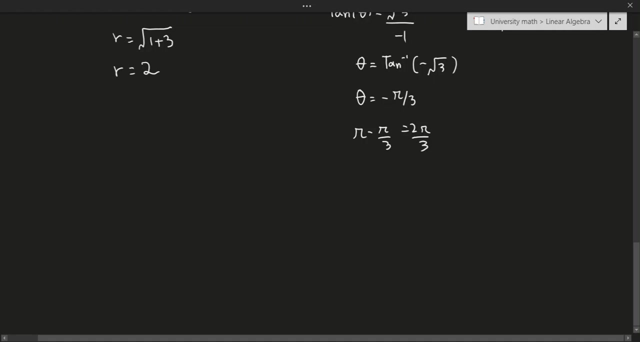 pi to this. So what we could do is pi minus pi over three, is two pi over three, because that'll rotate this angle up there, which is kind of what we need. So, as a result, the equivalent angle that we can work with is two pi over three. Okay, so that's really good. So that means we know the 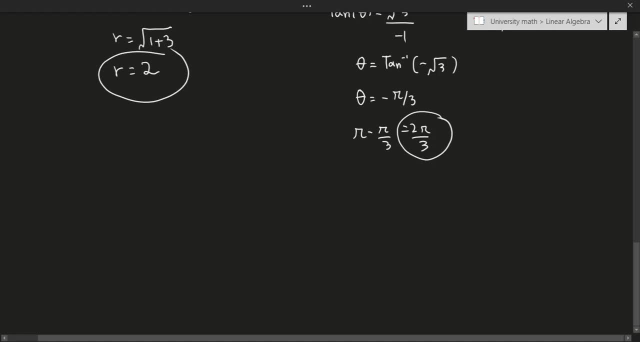 angle, which is two, pi over three, and we know the magnitude or the length, which is two. So that means in polar form our angle or not the angle, but the complex number can be rewritten as the following, So we can write this as two: 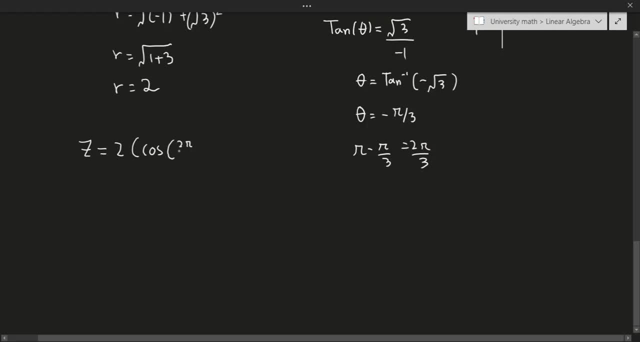 times cosine of two pi over three, plus i times sine of two pi over three. And that, right, there is our answer for this particular complex form. So not too bad. Okay, now let's do one more example of this. it'll be exactly the same kind of method, but for different numbers. So this one says: write: 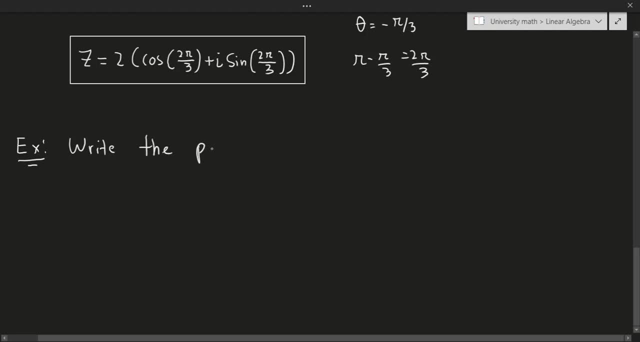 the polar form of the following number- it's going to be z- equals one plus i. Okay, so if we go ahead and calculate the modulus or the length or the magnitude, whatever you want to call it, that's equal to the square root of one squared plus one squared. there's nothing in front of i, so that's assumed. 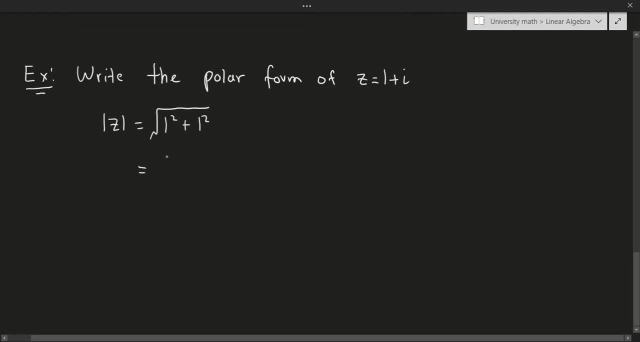 to be one, So that's going to give us the square root of two. Okay, so now let's calculate the bemol, So that's equal to the imaginary part over the real part, or Br a, So that's 1 over 1.. So that 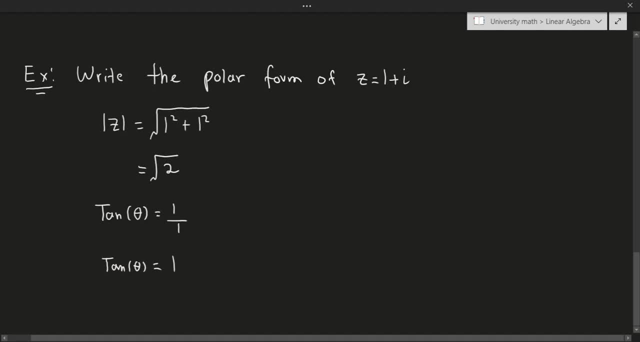 gives us one, obviously, because one over one is this one. And then teta equals tan inverse of one, but tan inverse one is pi over four. And this time pi over four is in the correct quadrant, because the vector, or not the vector, but the complex number one, if you would have thought, is going to be one. So this sine and then square root of two. we're just going to write that down to one. And then the n times one squared by one squared equals n squared, And that's what we have here. It's going to be two. So 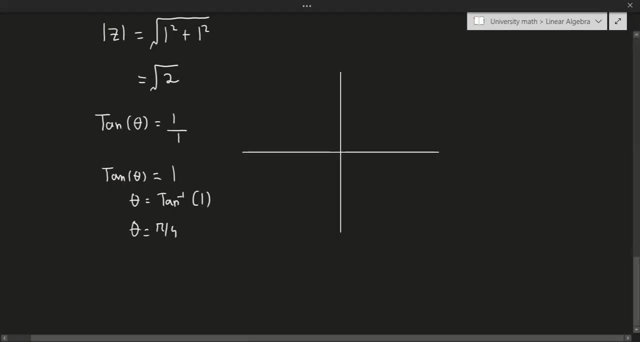 that's one squared over two, So that's equal to one over three. And then, if we go ahead and calculate, the 1 comma 1 is right there. So that's one, that's one and that's root two. So as a result we 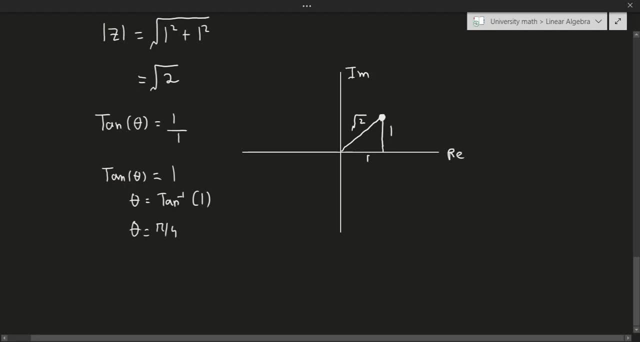 are in the correct quadrant, So there's nothing to worry about here. So now let's go ahead and convert this into polar form. So we know the magnitude and we know the angle. So we're going to get z equals root two, cosine of pi over four, plus i sine of pi over four. And well, that's our. 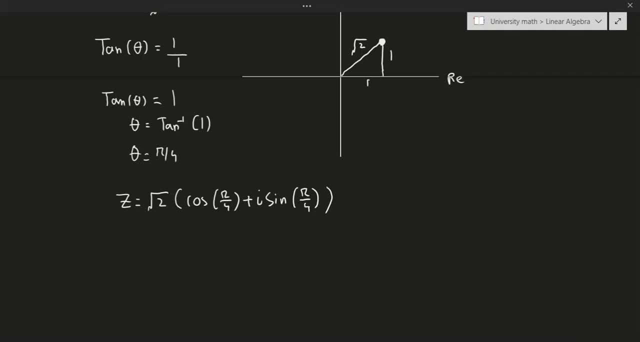 answer for this complex number in polar form. So let's go ahead and just oops, that's a circle. let's go ahead and box that answer. Okay, now let's go ahead And talk about exponential form. So exponential form is a lot more useful. 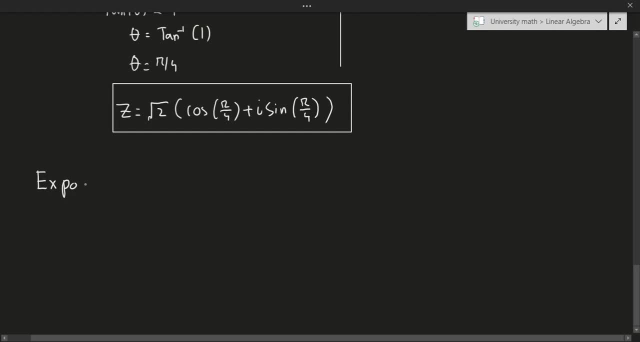 just because it lets us do a lot more things significantly easier. So exponential form. So let's talk about what this is. So exponential form uses Euler's formula, or Euler's formula, depending on how you pronounce it. I mean, I sometimes interchange it between the two pronunciations, but I digress. 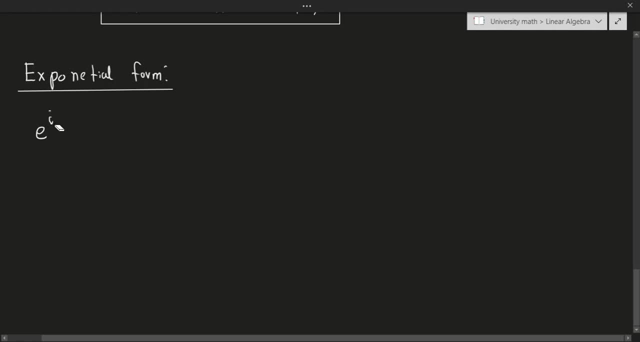 So Euler's formula says that e to the i theta is equal to cosine of theta plus i sine of theta. this is a very famous formula that's kind of. that was kind of developed by him, I believe. I don't know if he's going to keep up with it or if it's any math for him, but it's one of them. 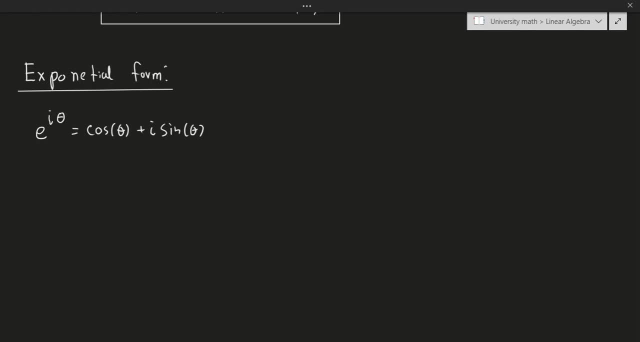 But regardless, this is one of the most famous formulas in mathematics And it's widely used in pretty much everything in complex analysis. So let's talk about how this is useful. We know the following: that z equals r times cosine of theta, plus i times the sine of theta. So we just go ahead and write this a bit better: i times sine of theta. 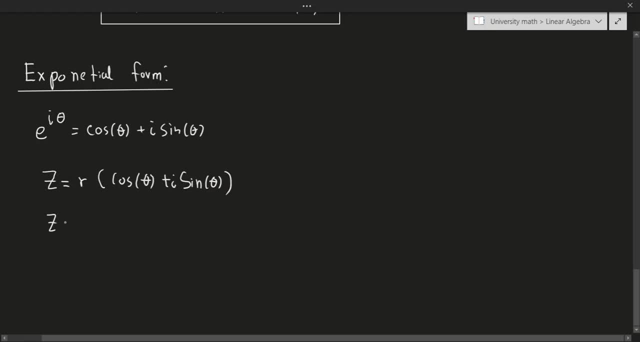 Okay, now recall that r is really just the length of z, And then the rest of it just stays the same. So let's go ahead and copy paste the exact same thing. So right there and right there. There we go, Okay. 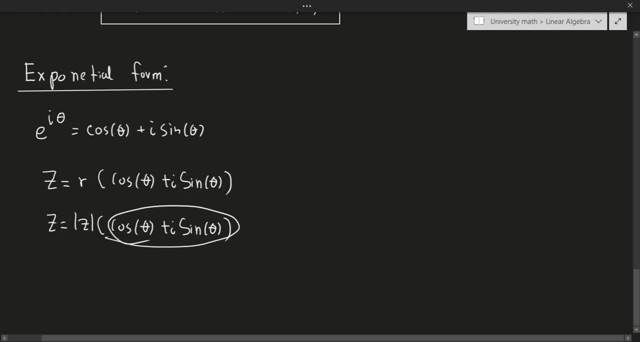 so now what's going on Is that? well, this part right there, if we kind of look at this part, is e to the i theta right there. So as a result, we get: z is equals to the modulus of z, or the length or the magnitude, whatever you want to call it, times e. to the i theta. So let's just go ahead and copy paste it and then we get z is equal to sine of theta, And then we get z. we get a to the i theta plus i times sine of theta. So, as a result, we get z equals to the modulus of z, or the length or the magnitude, whatever you want to call it- times e to the i theta. 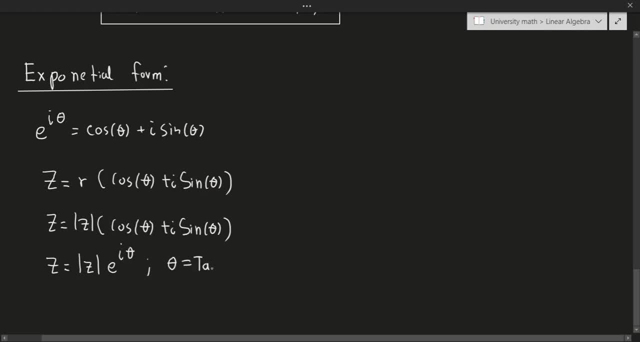 as usual, theta equals tan inverse of b over a. So this is just as before, So nothing different about this. And this, right there, is known as the exponential form of a complex number, So let's go ahead and box that answer. Okay, so this is known as the exponential form. 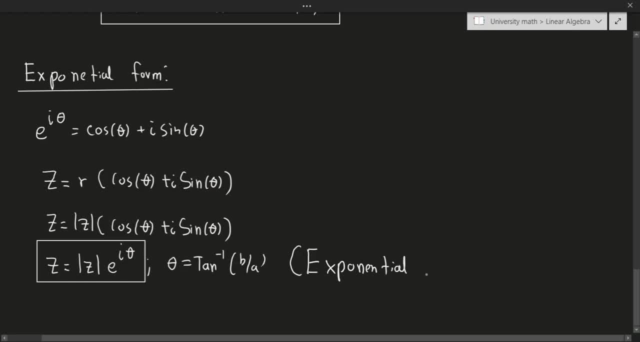 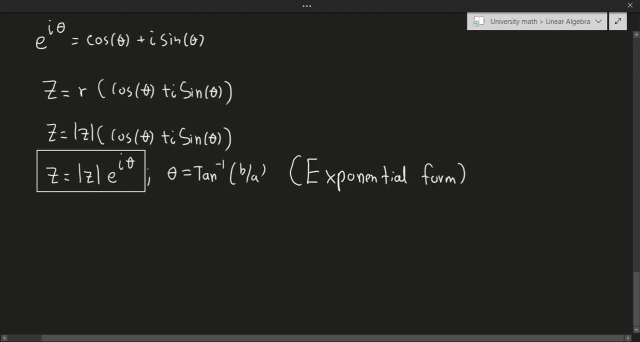 Like so. So very useful format for complex numbers, which we'll see shortly. So let's talk about why this is useful for a second, But for that let's just kind of do an example of just working with this complex number. So we'll do two examples of this. So write: z equals one minus root. 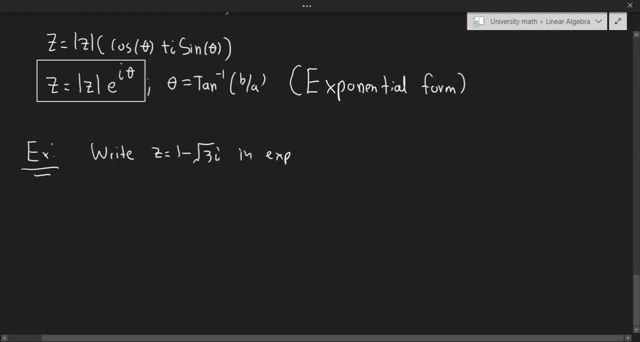 three times i in exponential form. Yeah, there we go. Okay, so how does this work? Well, we still need to calculate the magnitude. So z equals the square root of one squared plus minus root three squared. So by definition, this is equal to one plus three. one plus three is four. square root of four is: 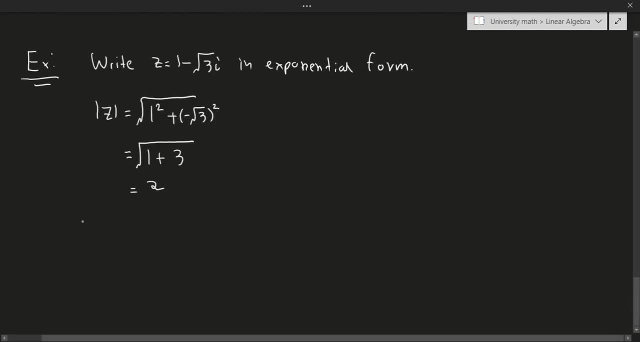 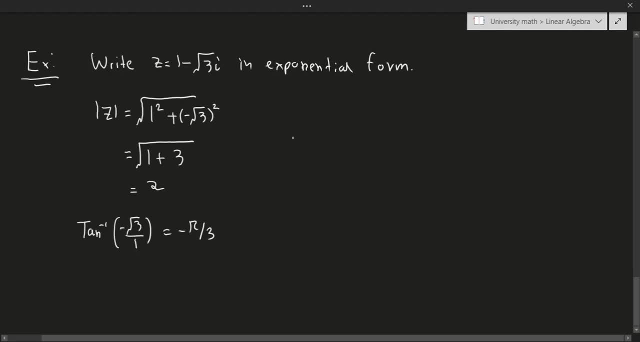 going to give me minus pi over three. And let's just plot this complex number just to make sure the angles are fine. So one minus root three, that's here. So everything is okay and the angle is fine. So that means in exponential form, z is equal to two, e to the minus i. 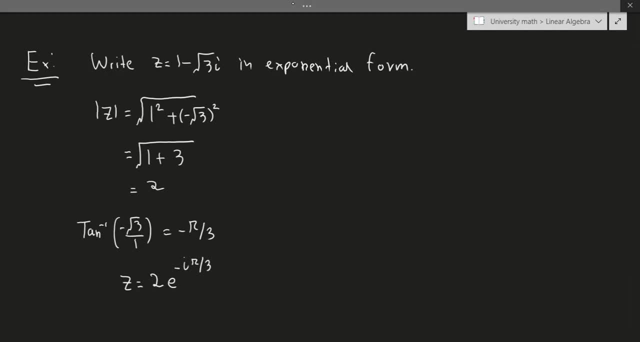 pi over three. this right there is equal to the exponential form of a complex number. So that's how this works. So let's talk about another, another example of working with this, And then we'll move on to a few more complicated and useful or practical examples. So let's just go ahead. 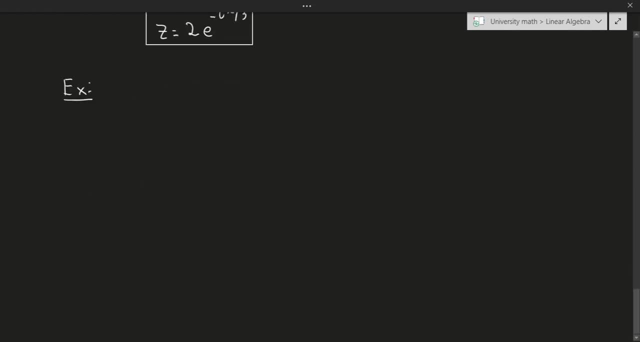 We'll just scroll up a little bit, just make sure we're covered. Here we go. Okay, so, okay. so now there's lots to work with this one. So right, z equals four minus four, i in exponential form. Exponential form. Okay. so how do we do that? Well, same thing. So we have to take the. 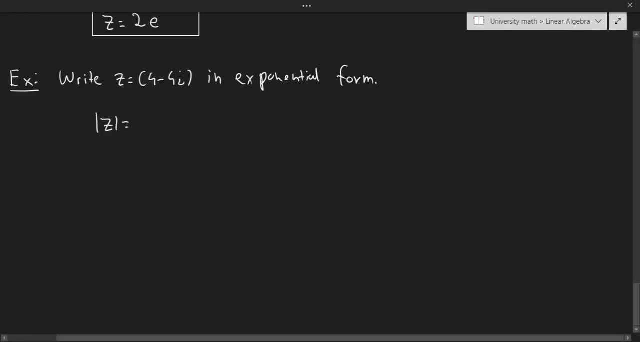 magnitude as usual. So z, or the magnitude of z, is equal to four squared plus negative four, all squared. Okay, so this is equal to four plus four times four, that's 16, or four squared 16.. That's also 16.. So we get the square root of 32.. This can be. 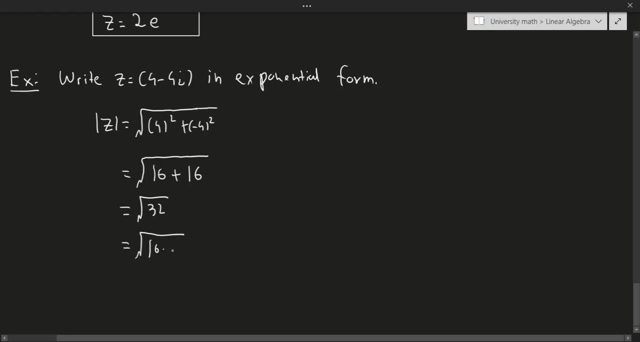 slightly simplified, because 32 is 16 times two and the square root of 16 is four. so we get four times root two. So that wasn't too bad. So now we just have to calculate the argument. So tan inverse minus four over four, Well, that's equal to tan inverse of minus one And tan inverse of minus one. 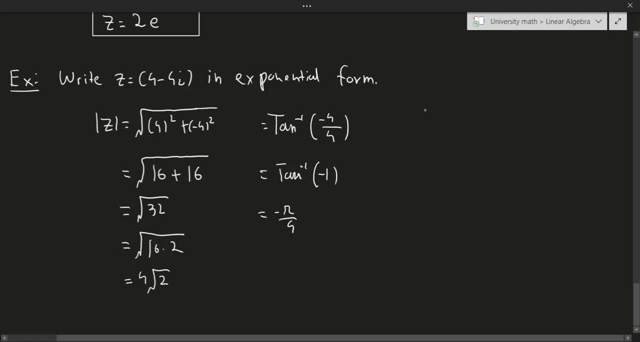 is minus pi over four, And let's just plot this complex number to make sure everything is okay. So four minus four, that's like here. So four minus four. So our angle is right there. So everything is okay. So this angle is valid. Okay, so now we have our argument and we have the magnitude. 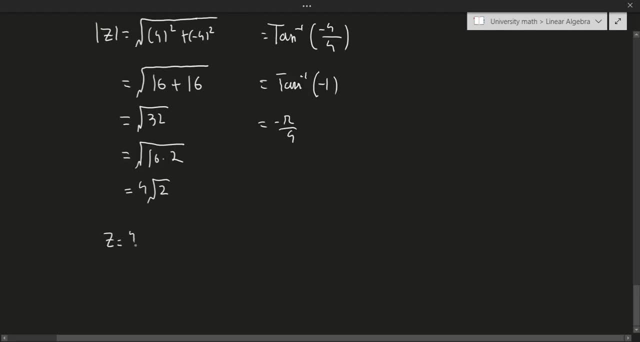 So that means z is equal to four root two, e to the minus pi over four times i. And that settles our answer with this question about how to calculate the complex or the exponential form of a complex number. So we're done with this example. Okay, now let's talk about why this. 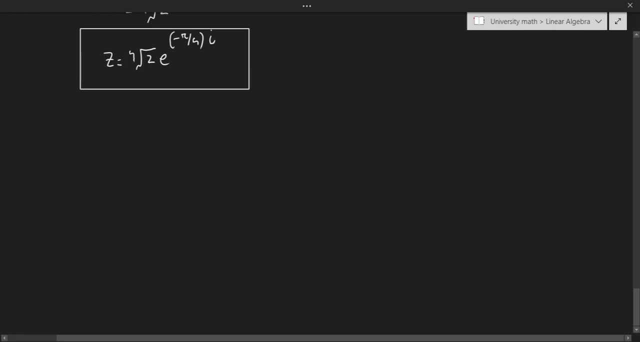 is actually useful. We can use this to calculate very large powers of complex numbers in a much more easy or an easy to understand kind of way. So let's talk about what I mean by this. Suppose I asked you to calculate well z, so compute. 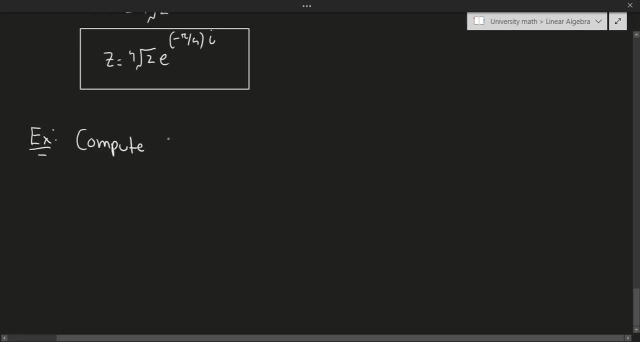 z, or let me just make this writing a bit nicer: compute z equals four minus four i to the power of 27.. Now, of course, you could, you know, just expand the life out of this and do it two times, But this would be extremely unpleasant. So let's talk about how to actually do this in a 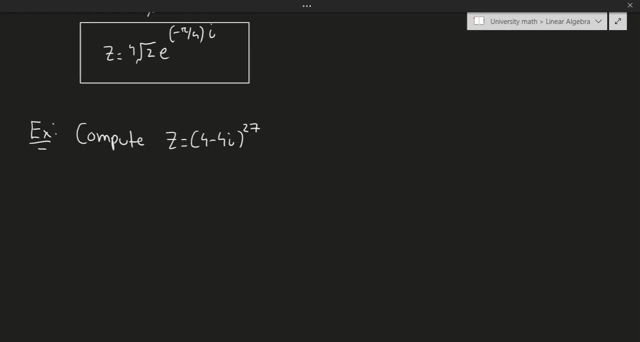 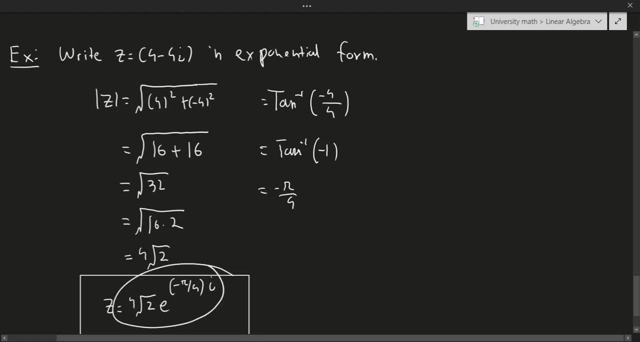 more nicer way. Okay, so if you take a look here, we already converted this thing into exponential form in the previous question, So let's kind of work with that. So in exponential form, z is equal to four root two, e to the minus pi over four times i. 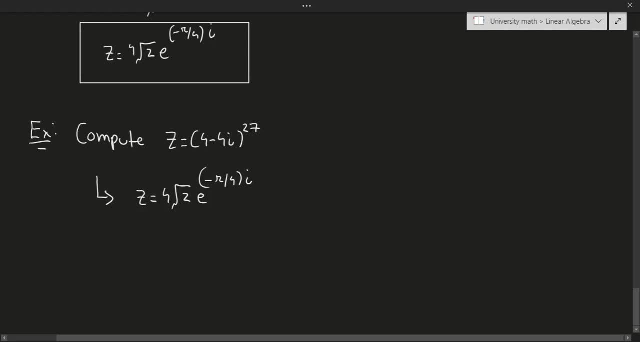 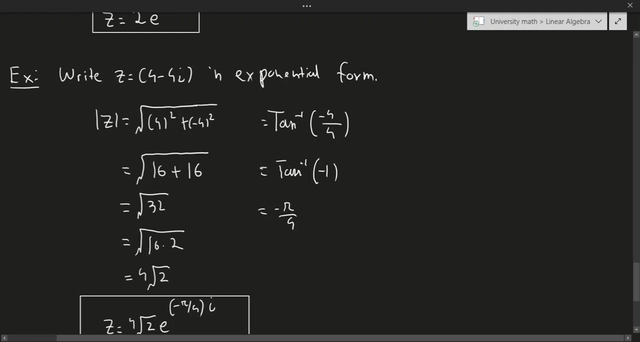 So why is this useful? Well, that means, by definition, z to the 27,, because we want to raise this to 27.. So, just to be very clear, this was just 4 minus 4i, So I could just raise the exponential form of this to the power of 27,, and we will be done. 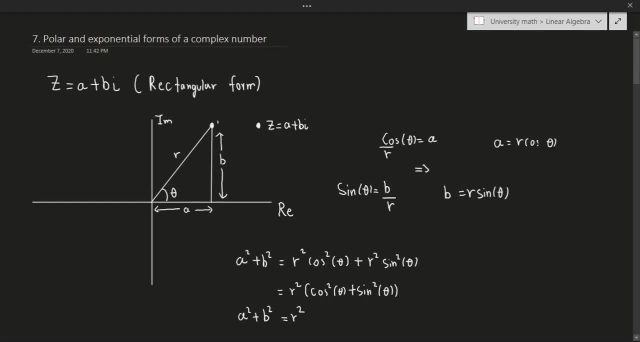 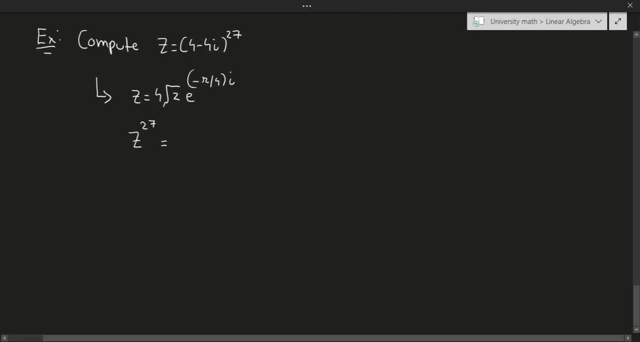 We just have to convert it back into rectangular coordinates or polar form as desired, when we kind of work with our, when we kind of finished off our simplifications, So let's talk about how this works. So z to the 27.. So that's going to be equal to four root two to the 27, e to the minus pi over. 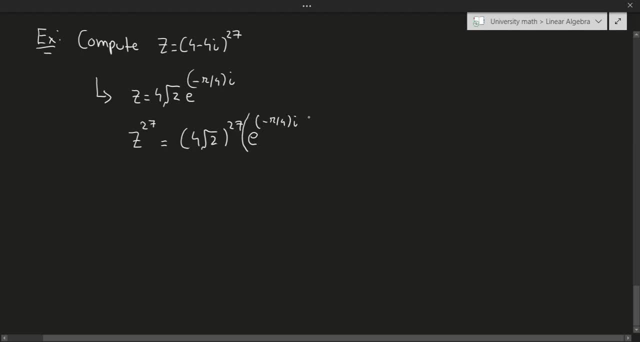 four times i to the power of 27.. Okay, so now what we can do is we can use our exponent rules, So you can write this as four to the 27 times root, two to the 27.. And then here we can write this as e to the minus 27 pi over four times i. So let me just go ahead and erase. 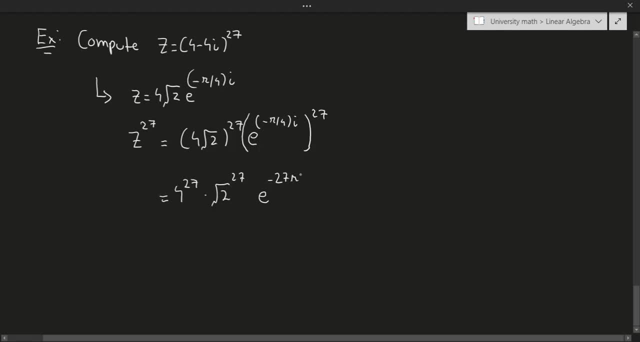 this pi over four times my, actually, because it's a bit nicer in general. e to the pi over four times i. Okay, so now let's talk about how to make this a little bit nicer. Well, four is the same thing as two squared, So we can write this: write this as two squared to the 27. 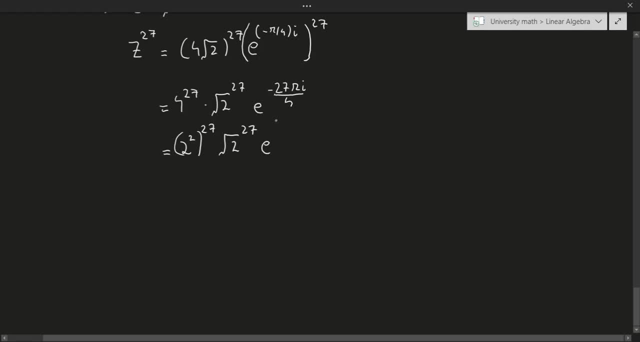 root two to the 27 e to the minus 27, pi i over four. Okay, so two to two to the 27.. So like that that's equal to two to the 54.. And then root two to the 27 e to the minus 27, pi i over four. Now here's the thing. 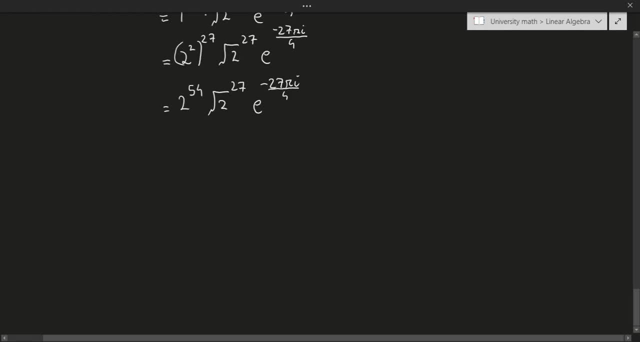 root two to the 27 can be slightly simplified because we can rewrite this as two to the 54 times root two to the power of 26 times root two, because that makes this an even power which is easier to work with times e to the minus 27 pi i over four. Okay, now we get two to the 54 root two. 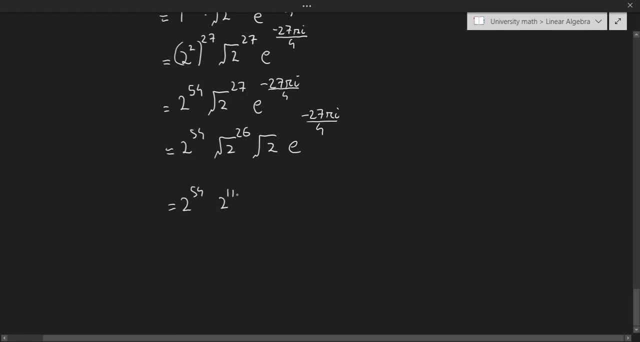 is the same thing as two to the one half. So we get two to the one, half to the power of 26.. But one half to the power of 26, like that is this going to be equal to 13.. So this is the same thing as two to the power of 13.. 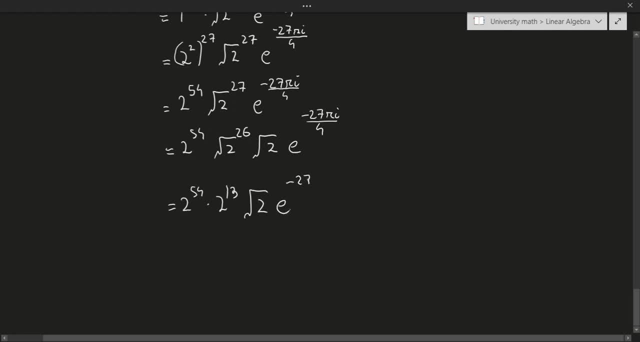 And then here we get root two e to the minus 27 pi i over four. Okay, so now how do we proceed with this? Well, one thing we can do is combine these two together. So this will give us two to the 67 root, two e to the minus 27 pi i over four. Now we can. 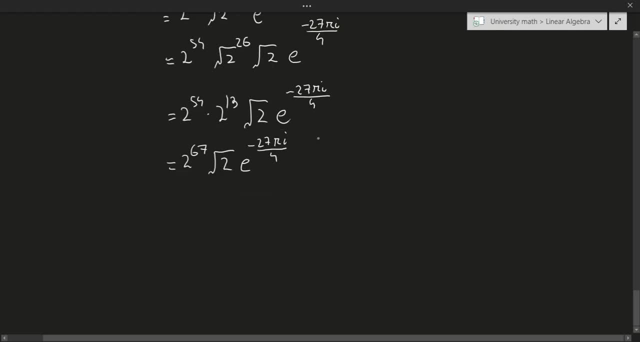 just convert this back to exponential, into polar form right away. But the angle minus 27 pi over four is a little bit unpleasant to work with. So how can we rectify this problem? So is there a way we could write this angle as a sum of two nicer angles? Yes, there is, Because we know for a fact. 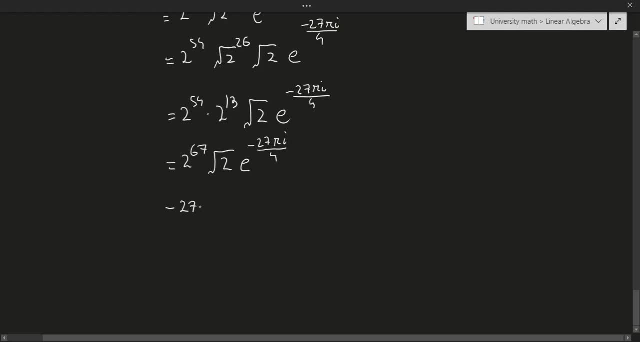 or if you do some, if you'd love a little bit of work, minus 27 pi over four is the same thing as to be pi over four. Firstly, f to a power of zero plus 37 pi plus zero, That is the sum of two decimals per four times prouds. 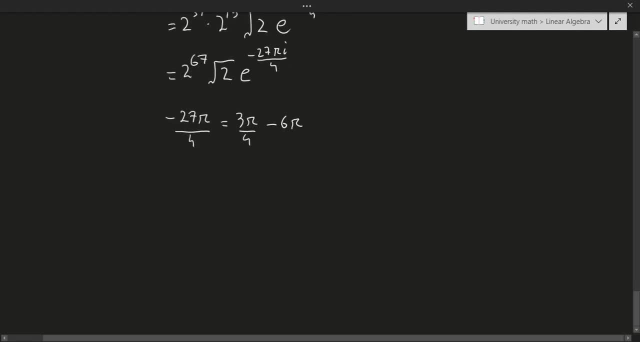 six pi, So this is significantly easier to work with. So now let's go ahead and talk about this. Okay, so this is equal to two to the 67, root, two e to the minus three pi over four. i- Yeah, I just let me, just because writing a little bit better: three minus three pi over four times i. 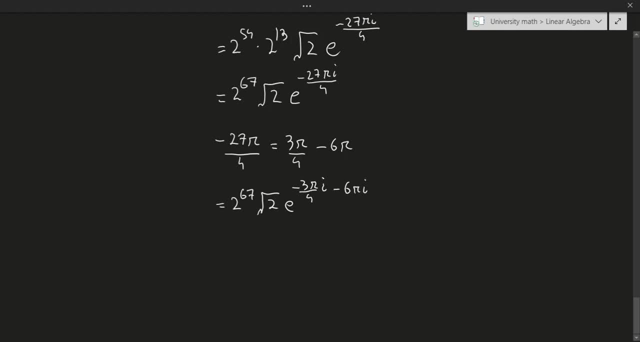 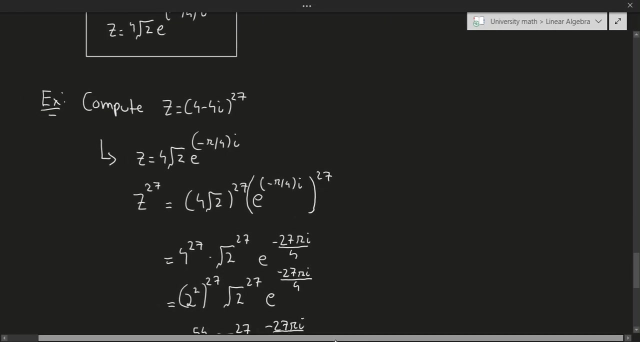 minus six pi i. So now what we can do is split the exponents apart, So let me just go ahead and move this over a little bit. Just make sure everything's consistent. Yeah, that looks okay. So make sure everything's consistent. 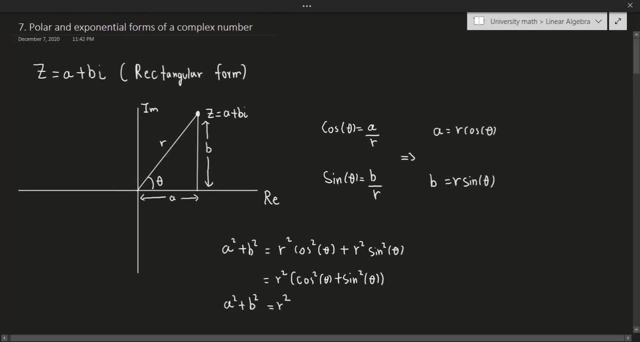 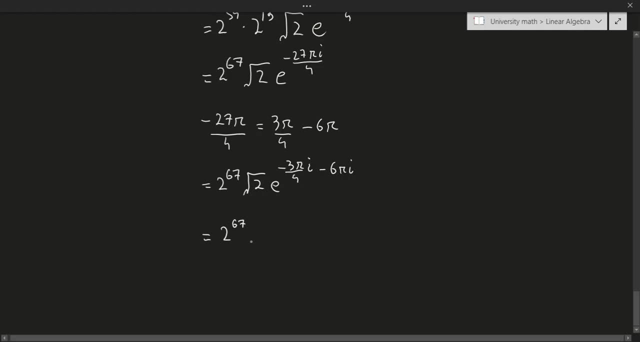 consistently spaced. Yeah, that's a bit better. Okay, now let's continue. So this is equal to two to the 67, root, two e to the minus three pi over four i times e to the minus six pi times i This. 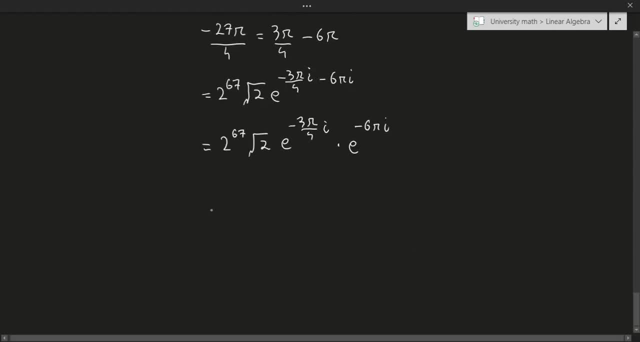 right, there is just equal to one, And the reason for that is because e to the minus six pi, i, by definition, is equal to cosine of minus six pi plus i times sine of minus six pi. But that's just equal to. well, this part is equal to: 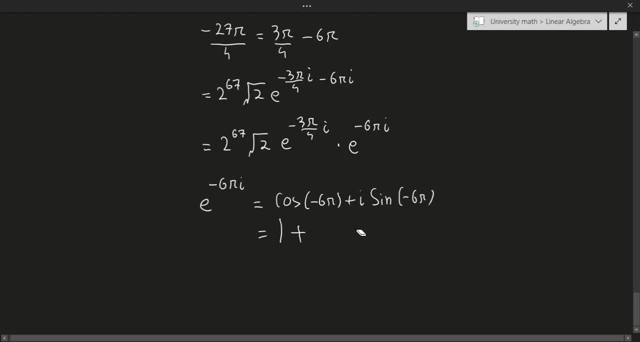 one And this part is equal to zero, because sine of six pi minus six pi is zero. So you get one plus zero or one. So all we're kind of left with now is two to the 67, root, two e to the minus three pi over four times i, And then this part is one. so we can just ignore that And 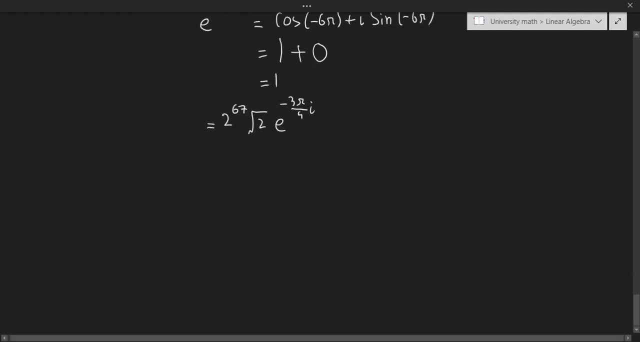 there we go. that takes care of this part. So now what we can do is convert this back into polar form, So we can write this as two to the 67, root, two times cosine of minus three, pi over four plus i. 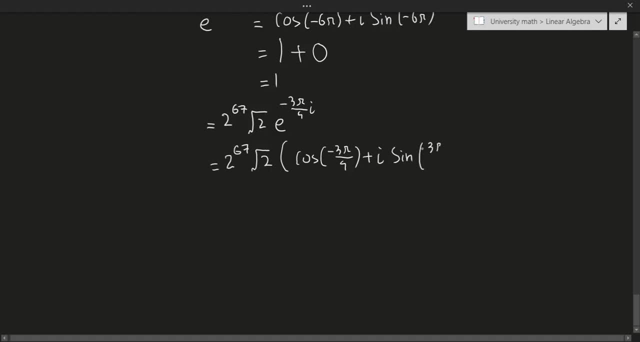 times sine of 3 pi, or minus 3 pi over 4, right there. So that's going to be equal to 2, to the 67 root 2 times. well, this is minus root 2 over 2 plus i, and this, right there, is minus root 2. 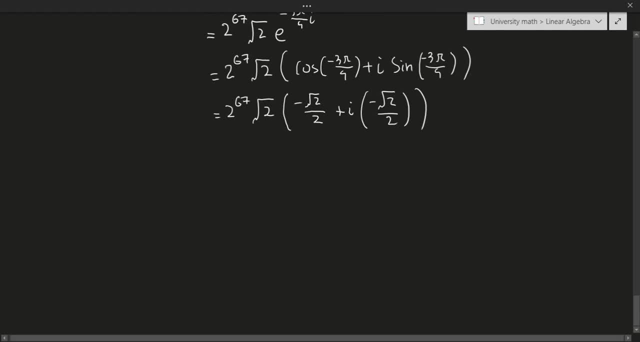 over 2.. Okay, so if we go ahead and expand this root 2 to both of these terms, we're going to get 2 to the 67 times minus 2 over 2, plus i times minus 2 over 2.. But minus 2 over 2 is just negative. 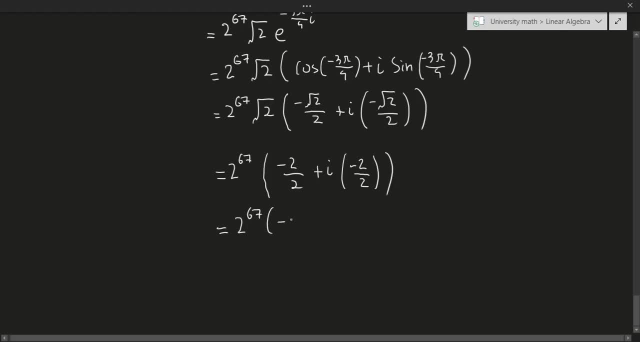 1, so we get 2 to the 67 times minus 1 minus i like so, and then we can factor the minus 1 out. so we get 2 to the 67 times minus 1 minus i like so, and then we can factor the minus 1 out. 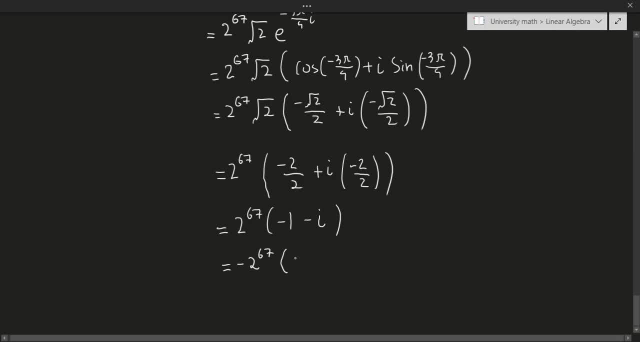 so we get minus 2 to the 67 times 1 plus i. Now we could, you know, evaluate 2 to the 67, but that's completely pointless. So now, technically, to write this in rectangular coordinates, we could write this as: minus 2 to the 67, minus 2 to the 67 times i, or equivalently. 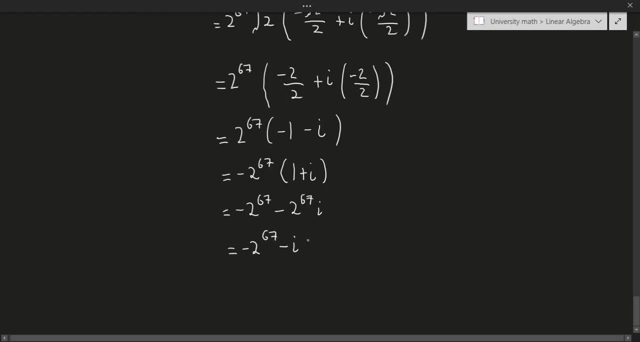 minus 2 to the 67. minus i times 2 to the 67.. It doesn't really matter which order you write it, but typically the first order is preferred. but some people prefer this method. It doesn't really matter per se, and that's how we calculate this answer. Notice how long this would have taken. 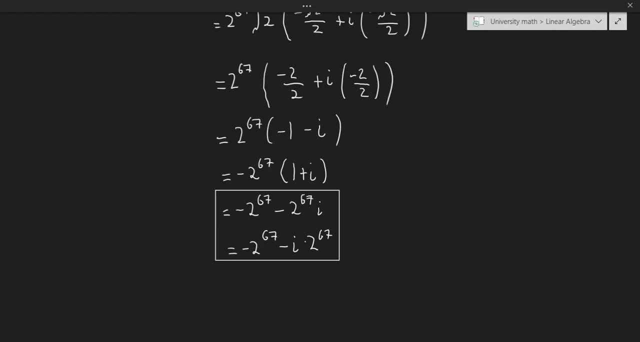 if you did this- the good, old-fashioned way of expanding this 27 times With the idea of exponential forms- this is significantly easier to compute and work with, so that's much easier and nicer to work with. as a result, Let's do another one of these examples. 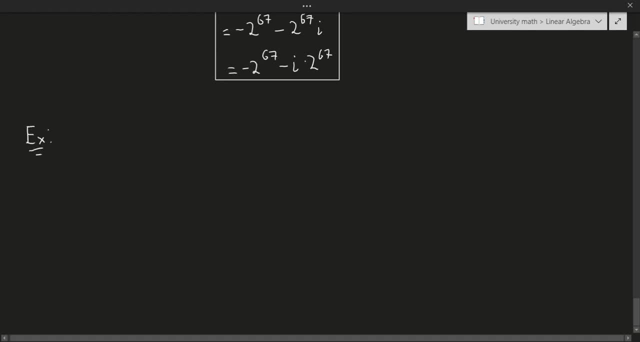 Just to make sure that we kind of understand this properly. So this one is compute 3 plus 3i to the 5.. Now, before I put a go on with this example, this is much easier to just do by hand. It is possible to expand this five times and then get your answer in a much more. 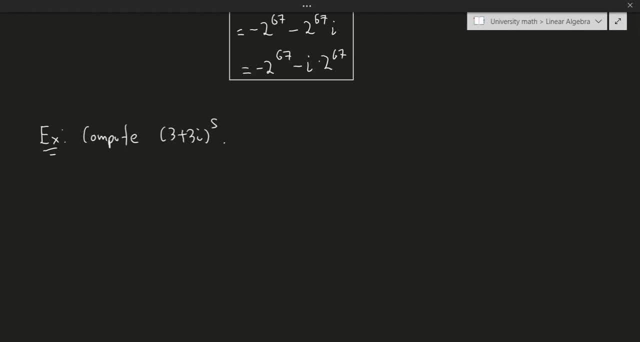 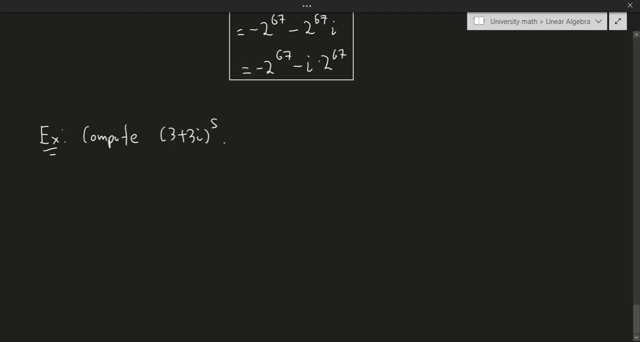 Let's do another one of these examples. Let's do another one of these examples. Let's do another one of these examples, But with the idea of exponential form. this is much easier to work with, So let's go ahead and calculate this using exponential forms. So the magnitude of z is equal to the square root of 3 squared plus 3. 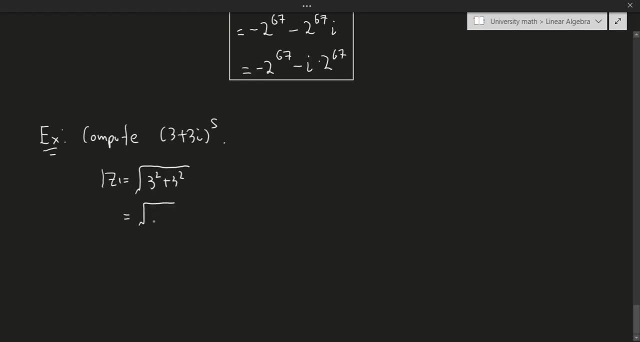 squared, but that's equal to 9 plus 9 or 18, and that's just equal to 9 times 2.. The square root of 9 is 3, so we get 3 times root 2.. Okay, so now let's calculate the argument. So the argument. 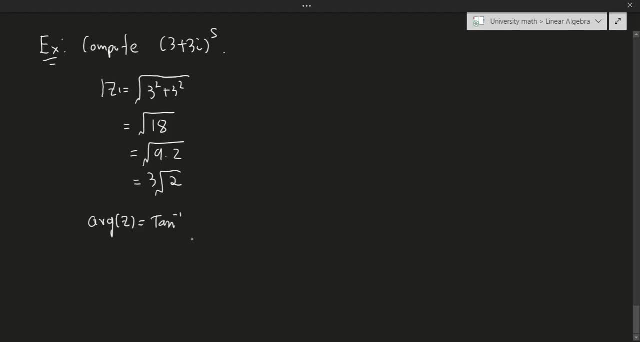 of z is equal to tan inverse of 3 over 3.. So we get tan inverse of 1, but that's just pi over 4.. And this is in the core quadrant, because 3 and 3 is just here. 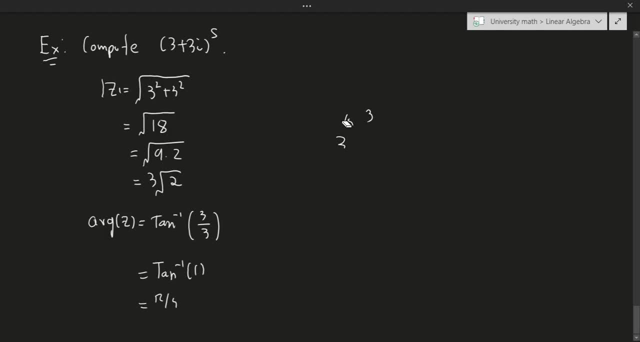 So we're okay, So there's nothing wrong with that. Okay, so now let's do another one of these examples. Let's go ahead and talk about this. So z, if you write it in exponential form, is 3 root 2 e to the pi, over 4 times i. 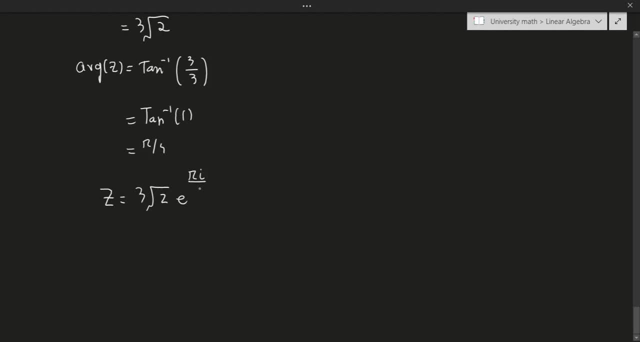 So let me just make this a bit better: Pi i over 4, like that. So just to be very clear at this point, we just computed 3 plus 3 i in exponential form, So you want to raise it to the power of 5.. Well, 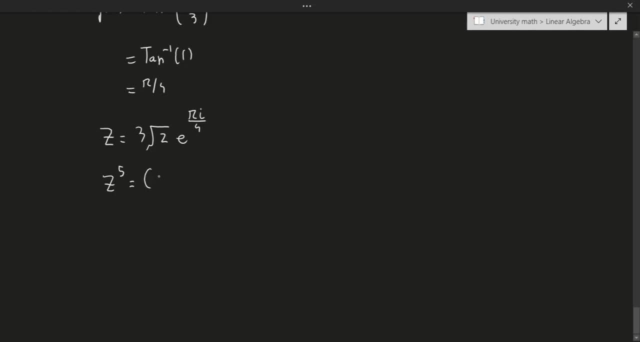 z to the power of 5, is equal to 3 root 2 to the power of 5, e to the pi i over 4 to the power of 5.. So this is going to give us 3 to the power of 5 root 2 to the power of 5, and that's going to give us e to the 5 pi i. 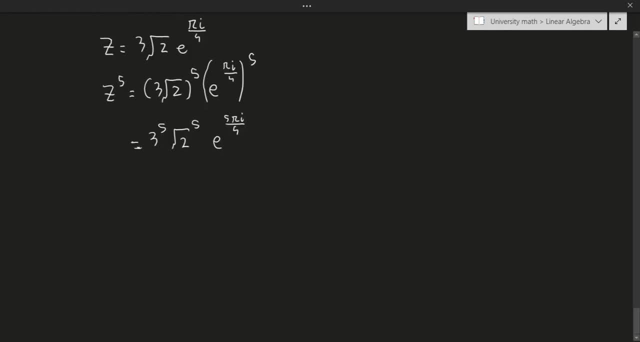 over 4.. Okay, so now what's going on? All right, So now, root 2 to the power of 5 is the same thing as root 2 to the power of 4 times root 2.. And that's going to give us e to the 5 pi i over 4.. Okay. 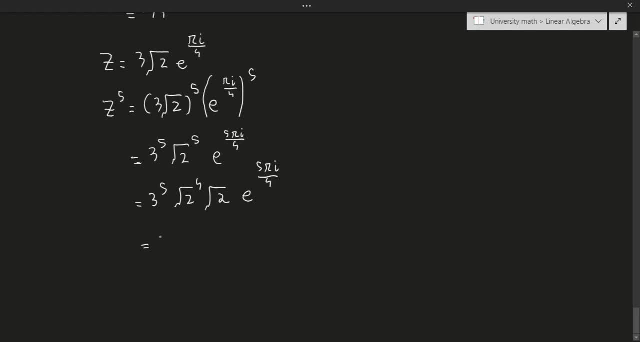 but root 2 to the power of 4 is the same thing as root 2 to the power. sorry, that's the same thing as 2 to the power of 2.. And then 3 to the power of 5, it's the same thing as. 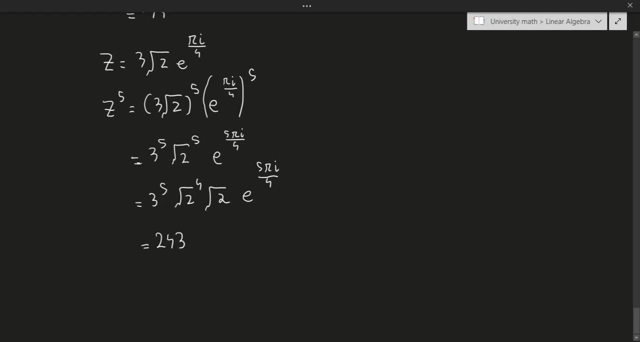 243.. So we get root 2 to the power of 4 is the same thing as 2 to the 1, half to the power of 2, so that's going to give us times 2 squared like. so then this gives us root 2 e to the. 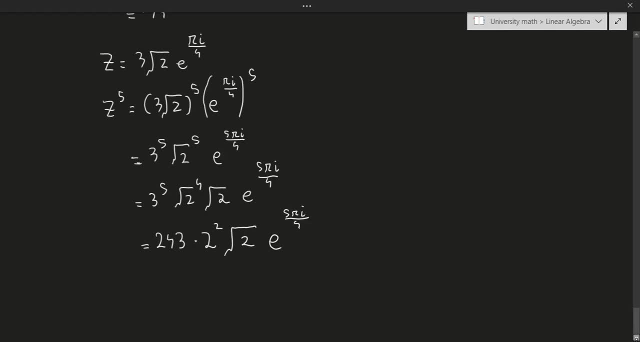 5 pi i over 4.. Okay now, 2 squared is 4, 4 times 243 is 972, so we get root 2, and then here we can convert this into rectangular form or not rectangular form into polar. 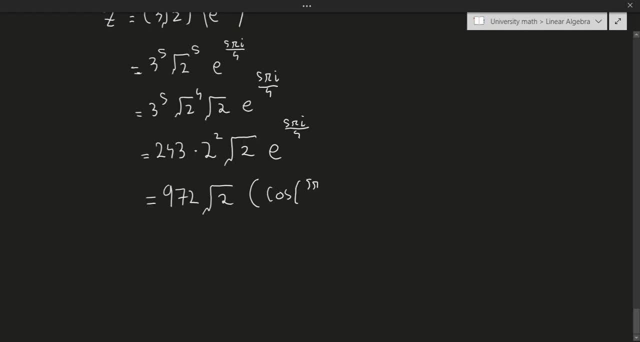 form. so we get cosine of 5 pi over 4, there we go, Plus i times sine of 5 pi over 4.. Okay, now this is not too bad to compute. so we're going to get 972 root 2, cosine of 5 pi over 4, that's minus root 2 over 2, plus i times sine. 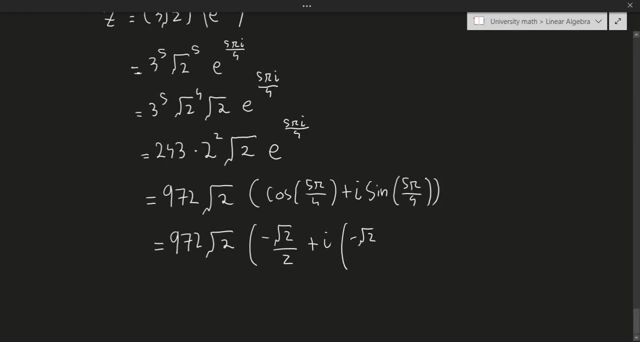 of 5 pi over 4, that's minus root 2 over 2.. So technically we can just put in the negative out and write like that. So if we continue doing our work, what we can do now is expand the root 2 inside all of this. so we're going to get 972 times minus 2 over. 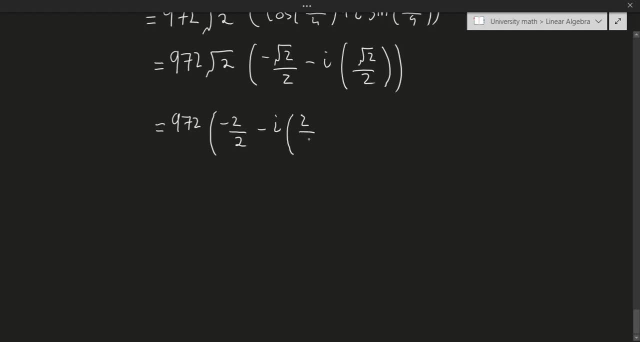 2, minus i times 2 over 2, like so, and then this is going to be 972 times minus 1, minus i like so, So not too bad. So now what we can do is we can multiply all of this by 972, so this: 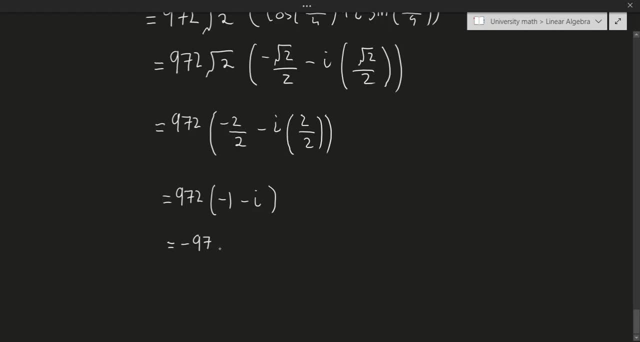 is going to give us minus 972, minus 972 times i, and that's going to be our final answer for calculating this with exponential form. So once again, we could have done this normally, but computing this with exponential form just makes things a lot nicer to calculate. Okay, 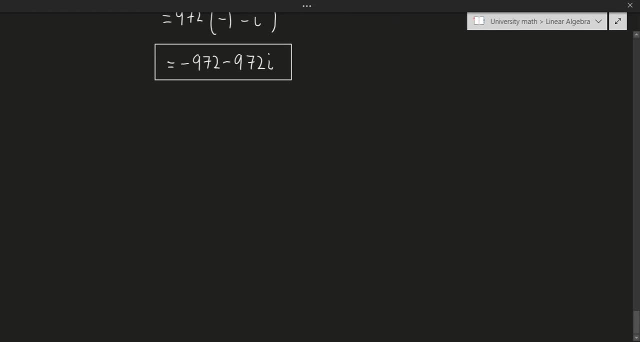 let's talk about another method, of why this is useful. We can also kind of perform complex arithmetic a lot more easier if we use the idea of exponential form. So let me talk about what I mean by that. So this is a rule, or some rules rather. So suppose I have. 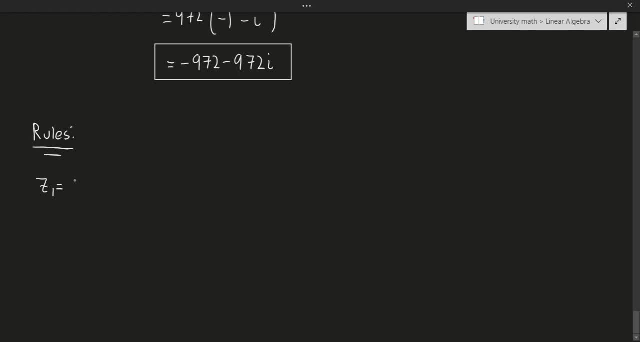 z1,, which is a complex number which is r? e to the i times theta. So this is an exponential form. And suppose I have another complex number, s, which is a complex number which is r? e to the i times theta. So this is an exponential form And suppose I have another complex number. 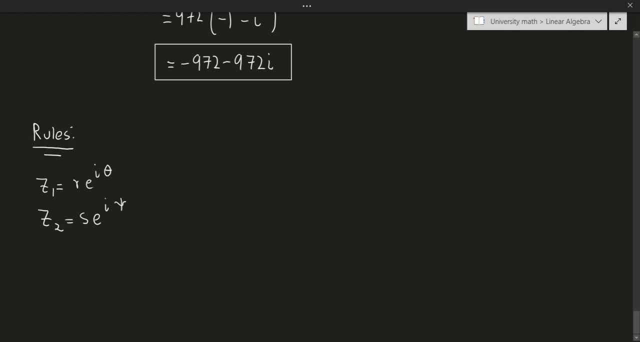 s e to the. i times some angle psi. So z1 multiplied by z2,. if I go ahead and multiply these, we'll get r times s e to the. i times theta plus psi. So instead of just you know. 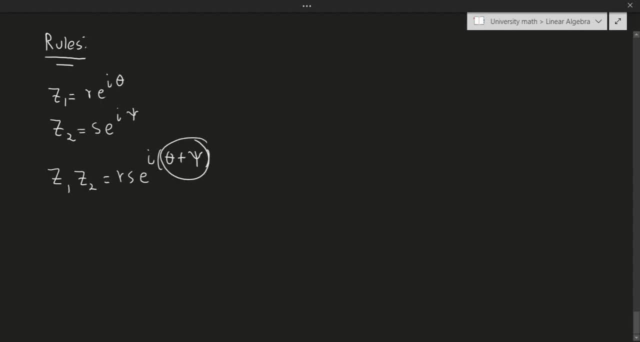 multiplying by using distributing property. we can just add the arguments together and get our answer that way, lot quicker than doing this normally using rectangular coordinates. So now let's talk about the same idea but division. So z1 over z2, in this case is equal to r over s, e to the power. 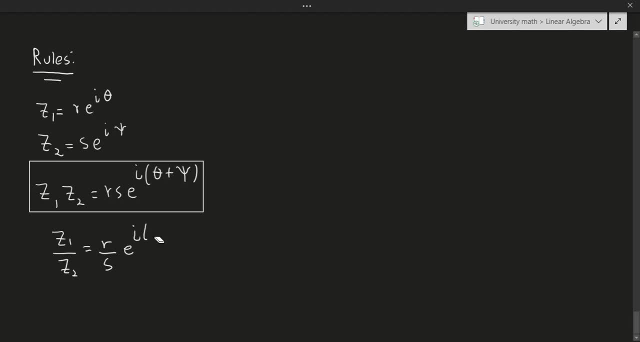 of i times theta minus psi. So let me just move this down a little bit like so, And let me just go ahead and make a rectangle out of this, And this will be our angle- or not our angle, but our rule- if we go ahead and divide two complex numbers. So 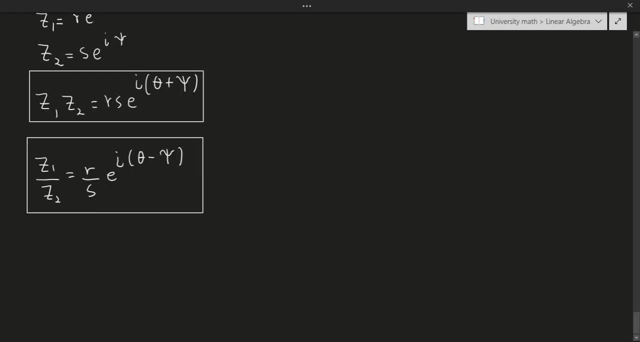 this will be our angle or not our angle, but our rule if we go ahead and divide two complex numbers. So there we go. Okay, so now let's talk about how this rule is useful. So let's talk about this example right here. So we'll switch back. So this one says compute the following: So compute root 3. 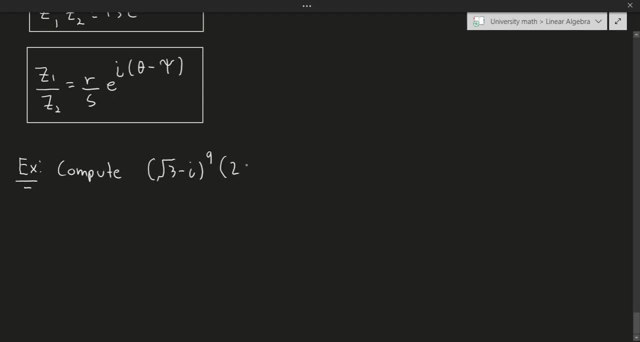 minus i to the power of nine times 2 minus 2i to the power of five. Now I think you can see the problem with this. I can, I can do it normally, But expanding this nine times and then expanding it. 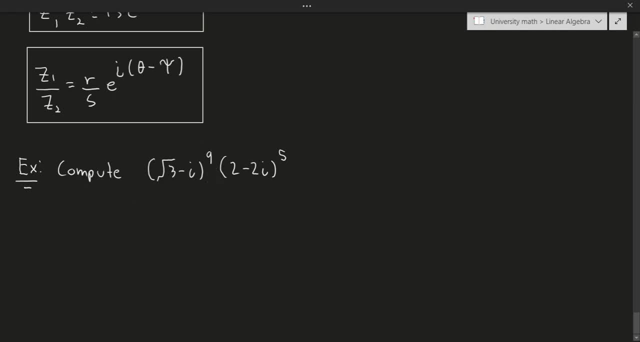 this five times. collecting all the like terms and then using this property will take a very long time. So it's probably an. there's probably an easier way to kind of compute this. So what we can do now is convert these both into exponential form. So let's go ahead and do that. So let's call. 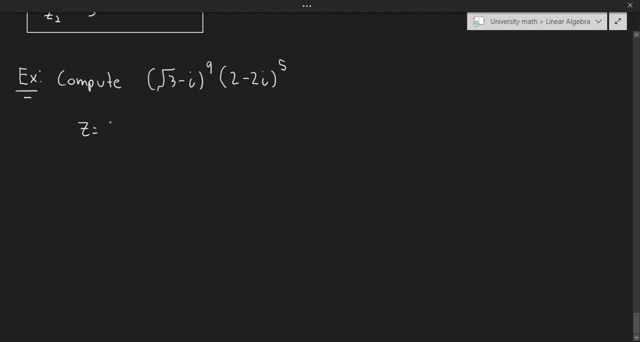 this number. So let's say that z equals root three minus i, and let's suppose that w equals two minus two i. So the magnitude of z equals the square root of root three squared plus negative one squared. Okay, so this is equal to three plus. 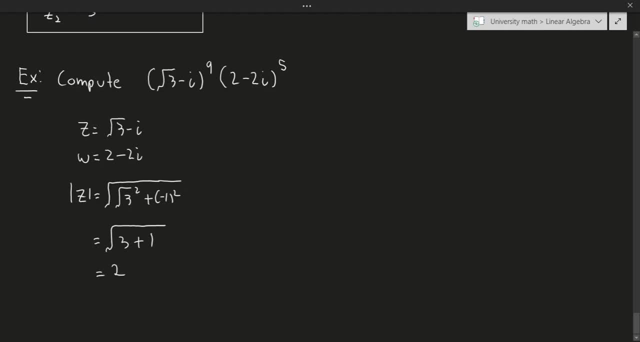 one p plus one is four. square root of four is two. Okay, now here we have this magnitude of w, So let's go ahead and calculate that. If you go ahead and do this, we get the square root of two squared plus negative two squared. So 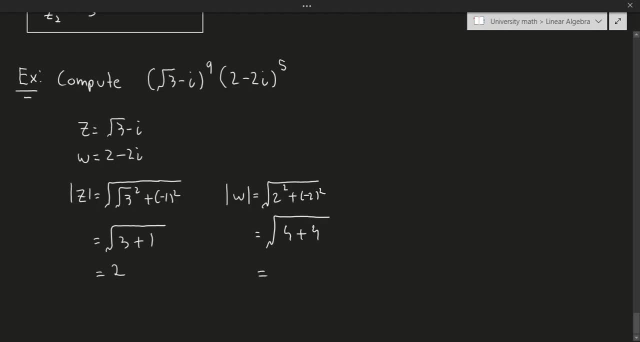 that's equal to four plus four And that's equal to root eight. But root eight, it's the same thing as the square root of four times two, And the square root of four is equal to two. so you get two times root two. So that's what we get, our, for our magnitudes, So for the arguments, so the 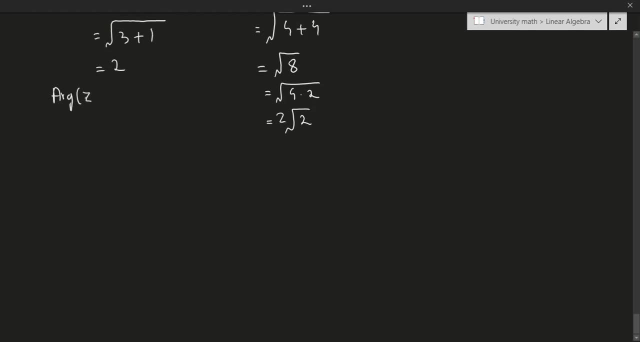 argument: z is equal to tan inverse of minus one over the square root of three. So that's going to give us minus pi over six. So that means for: in exponential form, we're going to get the following: So z is going to be equal to two e to the minus i, or- let's make this very clear- it's going to be two. 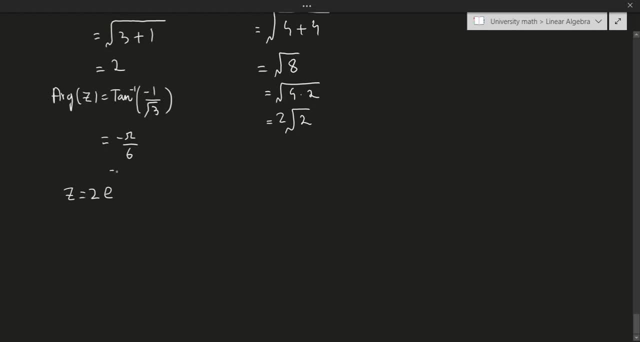 e to the minus pi, i over six, And then this one. well, we get to see if we get a similar kind of result. We know the magnitude, it's this, we know the argument, So let's go ahead and we don't know. 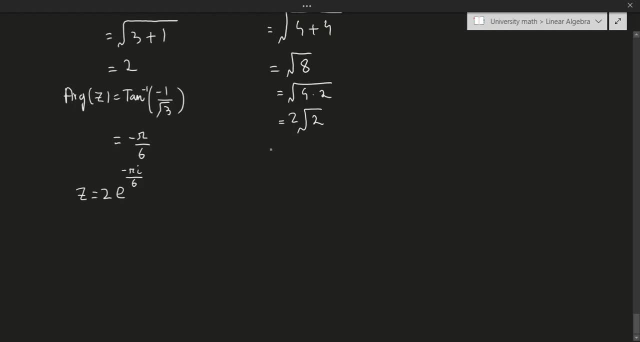 the argument. we're going to calculate that, Sorry. So the argument of z in this case is not z, w in this case is going to be equal to tan inverse minus one over two. So that's going to be equal to, sorry, not minus one over two, it's minus two. 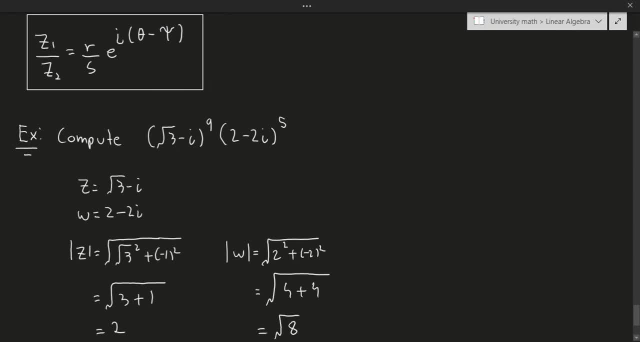 over two. So just making sure, that's okay. So minus two over two, Yep, that's fine. So let's go back down. So this gives tan inverse of minus one, or minus pi over four, And that's going to give us 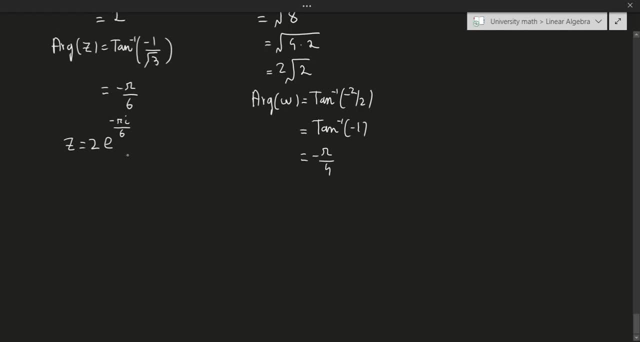 the following. So that means in this situation. so we're just going to underline this one. This time we get: w is equal to. let me just write that down. So w is equal to. let's see, it's going to be two. 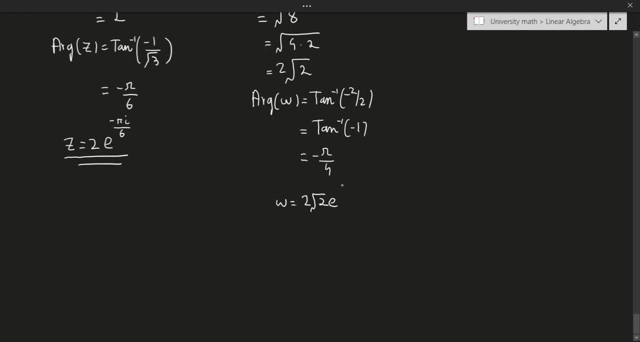 root two e to the minus pi times i over four. So let me just move this down a little bit, Okay, so that right, there is going to be our both of our complex numbers in exponential form. Okay, so this is significantly easier to work with. 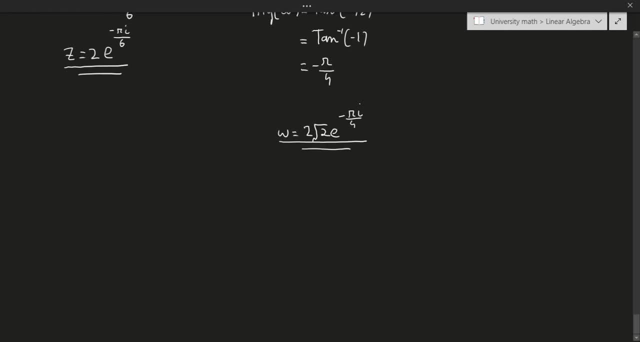 So let's go ahead and actually calculate these out. So z times w is going to give us three minus i times two minus two i. So that means z to the power of nine times w to the power of five is going to be three minus or not three minus i, it's going to be root times two. 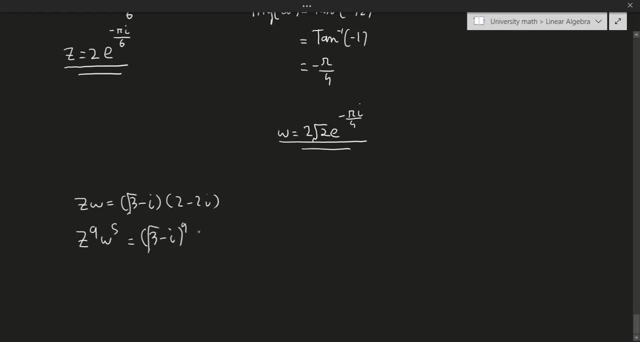 Yeah, there we go Root: three times i to the nine times two minus two i to the power of five. Now, once again, we're not going to actually expand this, because that will take forever, So what we can do instead is use the exponential form which we just calculated a moment ago, right? 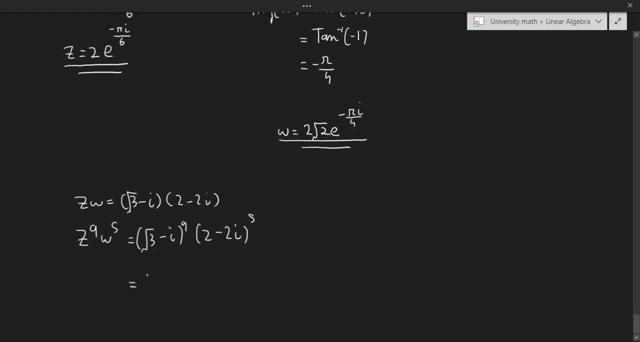 here. So if you go ahead and do that, well, let's take a look. Well, we're going to get two e to the minus i pi over six, To the power of nine times two root. two e to the minus pi i over four. 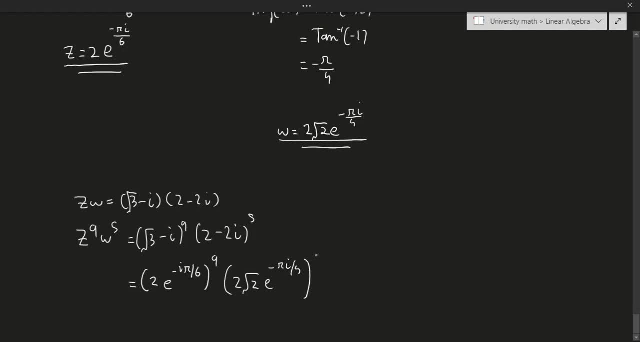 We just erase that tiny bit to the power of five. Okay, so that's what's going on there, So let's keep going with this. So now, if you go ahead and expand all this out, you'll get two to the power of nine. 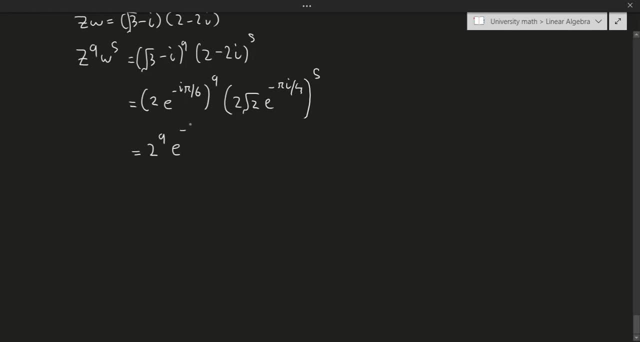 e to the minus nine pi i over six, And that's going to be times two to the five, times root, two to the power of five. e to the minus five pi i over four. Okay, so this is a lot nicer to kind of work with. So let's see what we can do Now. what we can do now is combine these two together. There's a lot of things that we can do here. So let's say that we're going to do this. So let's say that we're going to do this. So let's say that we're going to do this. So let's say that we're. 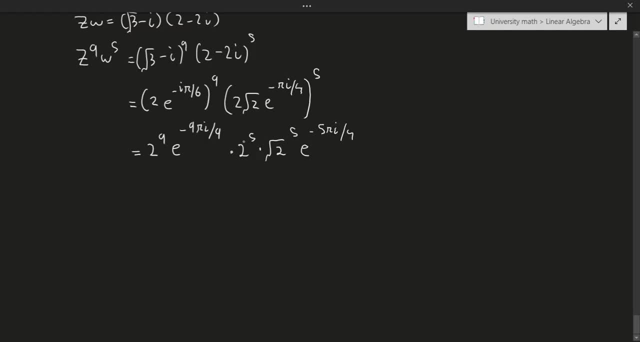 only one square root, so we can kind of work with that And then we can add these exponents together. So if we go ahead and do that, we'll get the following situation: So nine plus five, that's 14.. So we're going to get two to the power of 14 times root, two to the power of five. 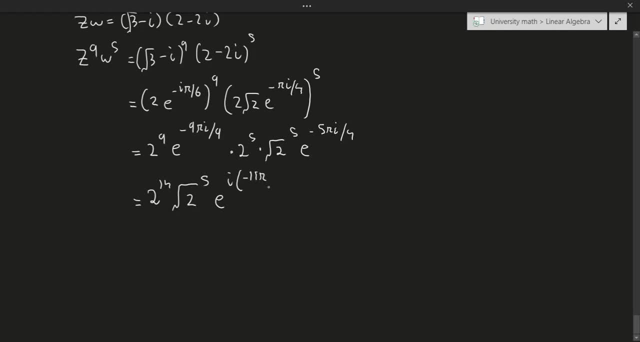 e to the i times minus 11 pi over four. So this, this part, just comes from adding these two fractions together. So let's go ahead and fix that writing a little bit. Okay, so now what we can do is the following: the square root can be dealt with a little bit. 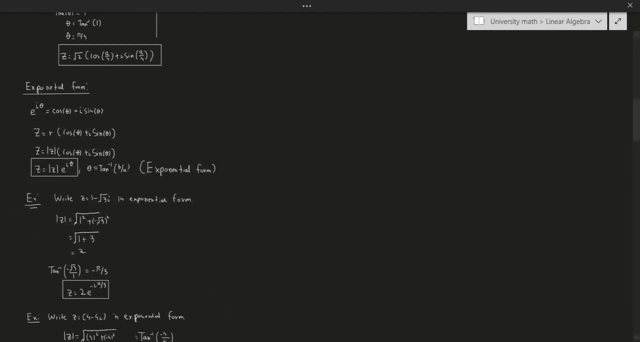 easier, So let me just go ahead and do that. Sorry, when I zoomed thing that was an accident. Okay, so just go back to normal. Okay, Yeah, that's a bit easier. Okay, so now what we can do. 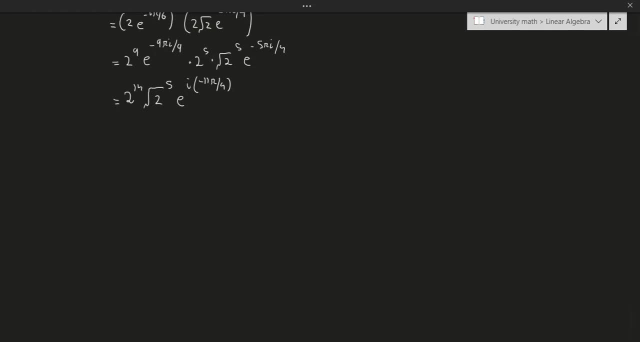 is the following: So root two to the power of five. So what we can do is write this in terms of an even power instead. So what we can do is write this as root two to the power of four times root two. And the reason for that is because, once again, root two to the power of four is going. 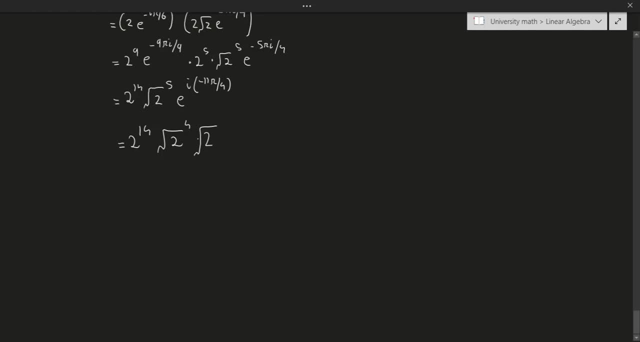 to be equal to two to the two and that's going to be equal to four. So that's a little bit easier to work with. This is still unchanged, So that's minus 11 pi over four. So that's going to equal to two to the 14 root. two to the four is two to the one, half to the power. 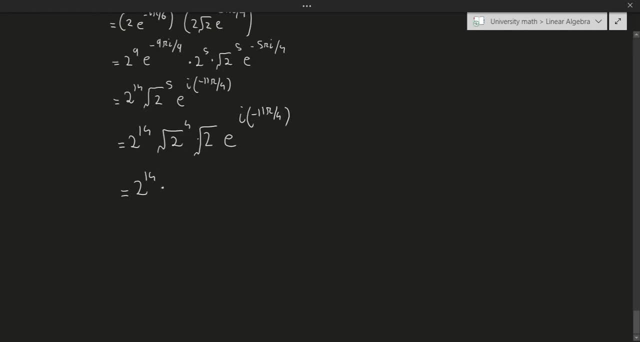 of four. So that's time. that's going to equal two times. Let's see two squared root two e to the minus. i times minus 11 pi over four. This is going to be two to the power of 16. root two e to the. 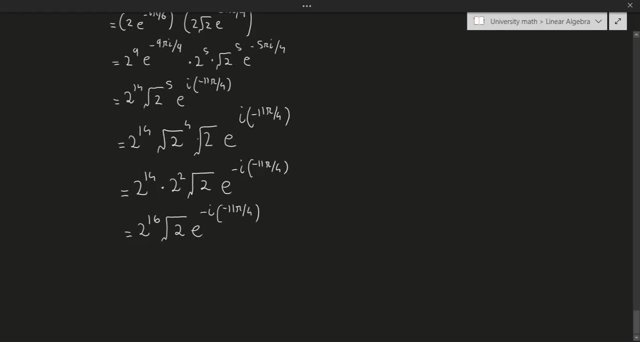 minus i times minus 11, pi over four. Okay, so now what can we do? Well, we can convert this into rectangular, or not rectangular, into polar coordinates, into polar form. So if you go ahead and do that, you'll get cosine of minus 11. 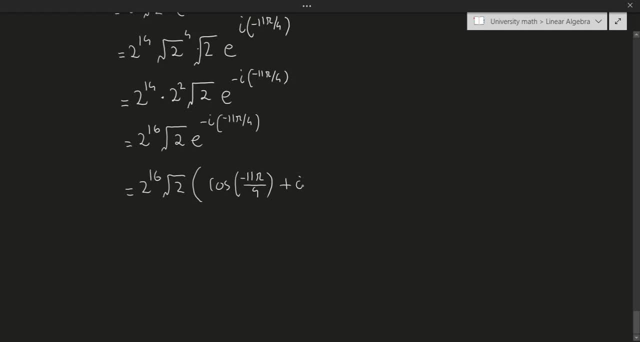 pi over four, plus i times sine of minus 11 pi over four. Okay, so now what can we do? we can calculate this using the unit circle. So if you go ahead and calculate this out, you look at minus root two over two, plus i times minus root two over two. Okay, 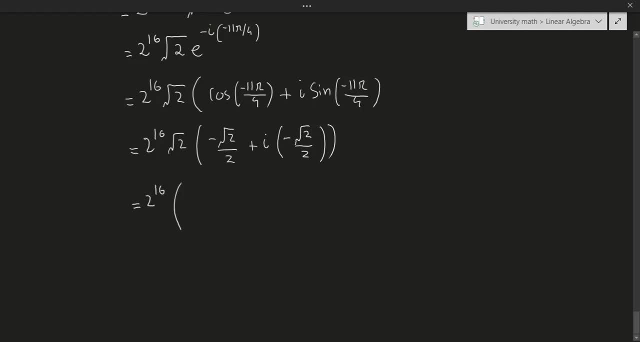 so now what we can do is multiply the root twos out, so we'll get minus two over two, plus i times minus two over two. but minus two over two is negative one. So we get two to the 16 times minus one, plus i times minus two over two, And then we get the conditional product of a constant of i. 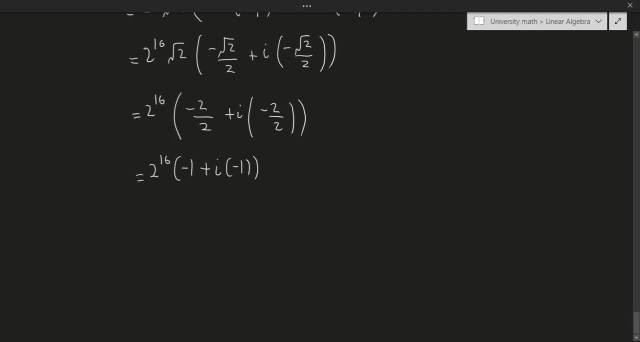 1.. Okay, so now what we can do is multiply the 2 to the 16 back in, So we'll get minus 2 to the 16, minus 2 to the 16 times i, or in other words, minus i times 2 to the power of 16.. Now 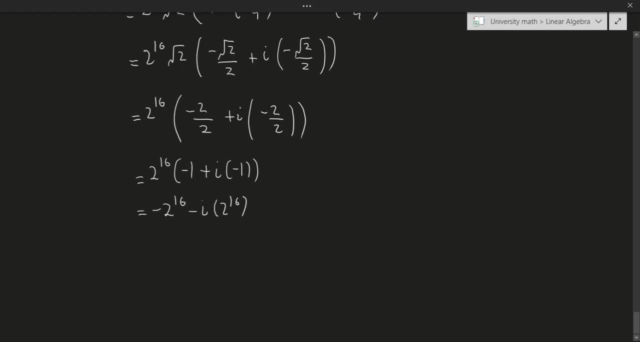 this is perfectly acceptable, But if you want to get the actual answer of this, if you really want to, this is equal to minus 65536.. So minus 65,536, minus 65,536 times i, And that would be our. 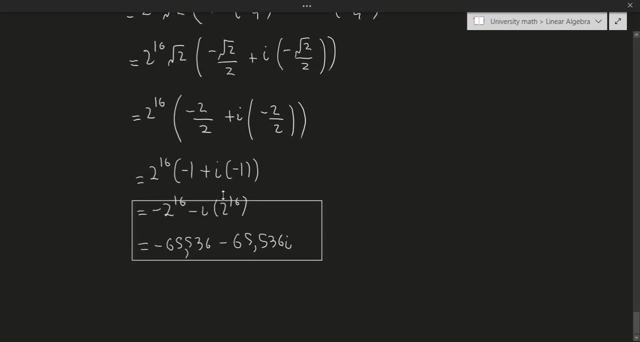 answer. This is a necessary because also the week we can leave it in this form. this is perfectly okay, But either one will give you the right answer. So that's how you calculate large powers using using exponential form. Okay, we'll do one more example involving trigonometry and trigonometric identities. 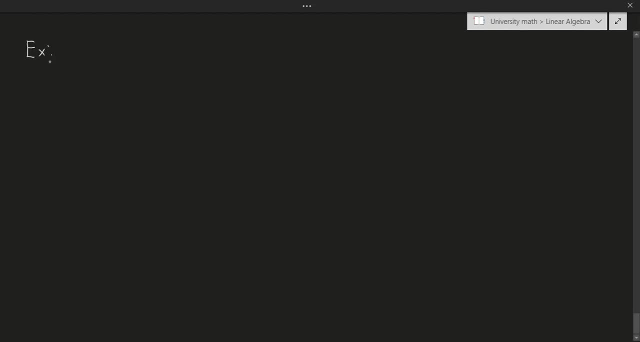 So suppose we want to do the following. So example: So use Euler's formula right here to compute the exact value of cosine of five pi over 12 and sine of five pi over 12.. Now I have to be. I have to note, five pi over 12 is not an exact value. 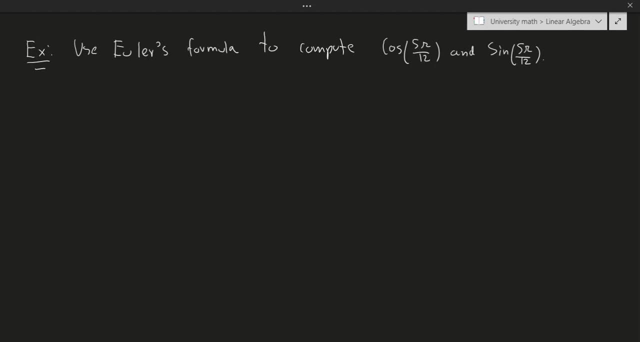 on any kind of unit circle or it's not. it's not kind of. it's not very easy to kind of work with numbers like this. So what most people usually do is rewrite this particular angle, given in terms of an angle that are in terms of sums or differences of 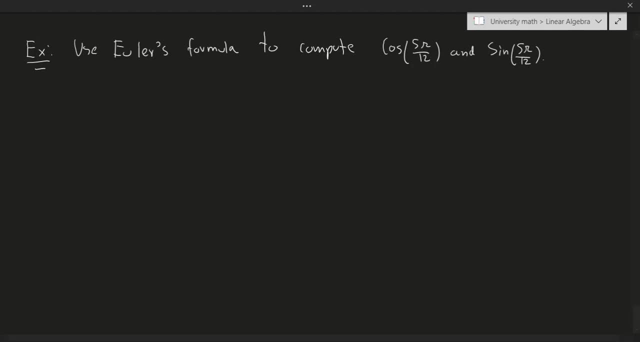 angles. they're easier to work with. So one thing we can do is kind of use the fact that five pi over 12 is the same thing as pi over four plus pi over six, because these angles exists on a unit circle and they're much easier to kind of work with. So let's kind 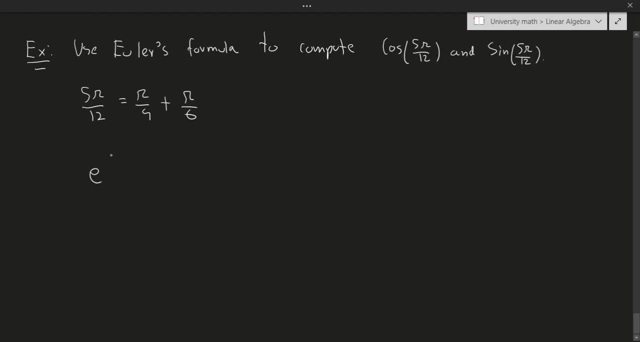 of talk about how to use this idea. Well, we know the following. we know e to the i times theta plus psi is the same thing as e to the i theta times e to the i times psi. But now we know what theta and psi are. So this is equal to e to the i times pi over four plus pi over six is equal. 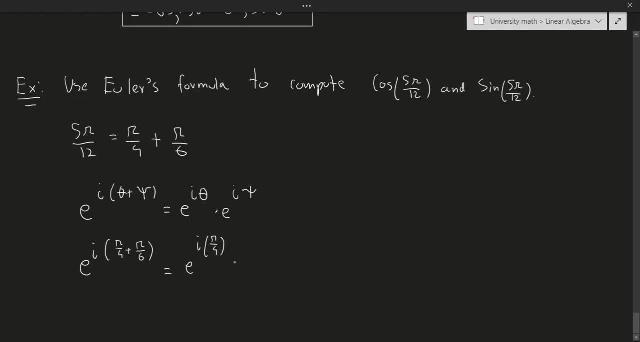 to e to the i times pi over four times e to the i times pi over six. So this is okay. So now, what can we do? Well, we're gonna get five pi over 12.. So e to the i times five pi over 12 is what we have here. 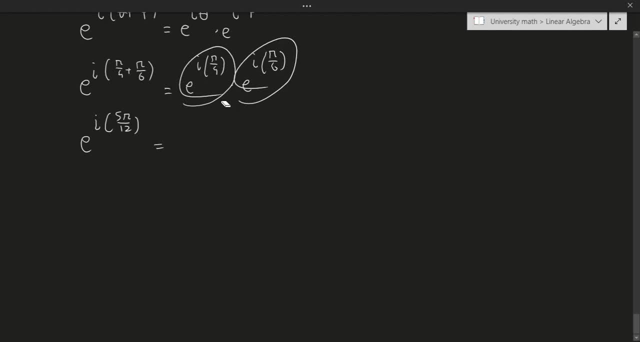 Over here. we're going to get the following, So we can convert these back into polar form: So if we go ahead and do that, we're going to get the following: is going to give us cosine of pi over four plus i sine of pi over four. Let's go ahead and erase that And then multiply. 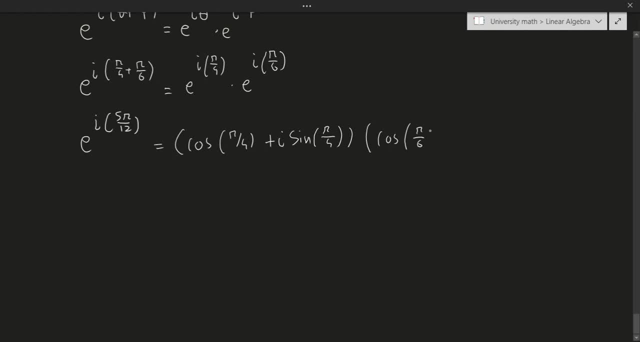 this by cosine of pi over four, of pi over six plus i times sine of pi over six. Okay, so the convert this back into polar form. we're going to get the following: So this is going to give us, so we'll just fix. 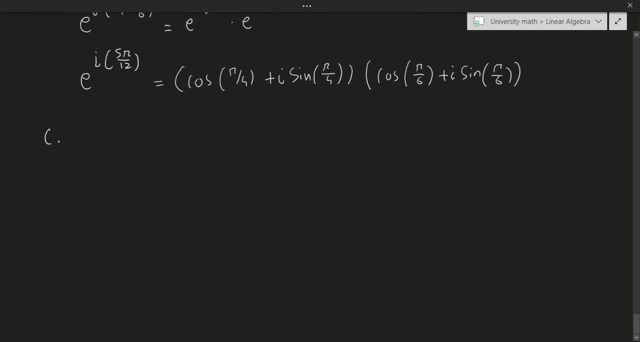 that a bit. So that's gonna give us cosine of five pi over 12.. Plus i times sine of five pi over 12.. Okay, so this part right there, that's gonna be root two over two, plus i times root two over two times cosine of pi over six, that's root three over two plus i times one half. 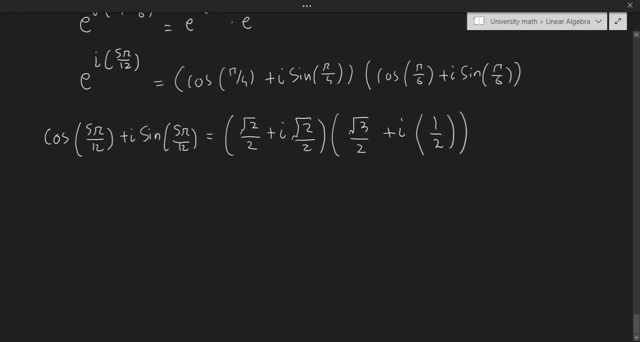 Okay, so that's going to be the situation that's going on here. So now let's talk about work with this mess. So how do we actually do this? Well, one thing we can do is expand this using the disappear property. So if we go ahead and do that, we'll get root six over four. that's. 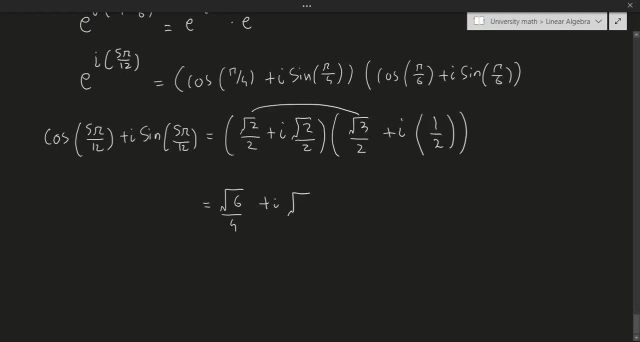 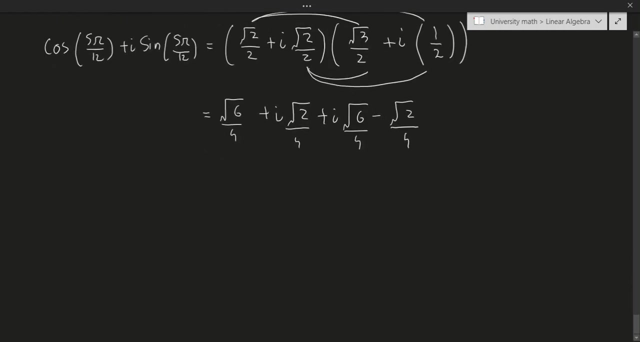 from here, plus i times root two over four that comes from here. Okay, here we're going to get i minus root two over four that comes from here. Okay, so now we can do. what we can do is kind of. 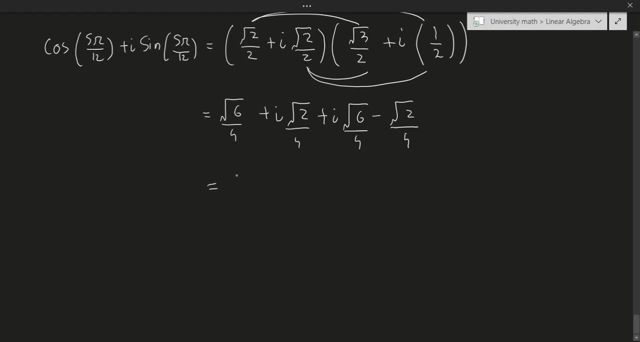 put these into rectangular coordinates, So we'll get mine root six minus root two or four plus i times root two plus root six over four. Okay, so now this means that we have the following: we have cosine of 5 pi over 12 plus i times sine of 5 pi over 12 is equal to the right-hand side. 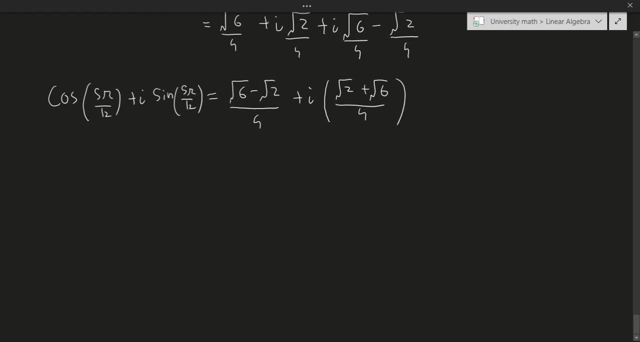 Okay. so what's going on here? What can we do? Well, what we can do now is we can equate the real parts, the imaginary parts together. So that means, by definition, cosine of 5 pi over 12 is going to be equal to root 6 minus root 2 over 4.. And if you equate the imaginary parts, 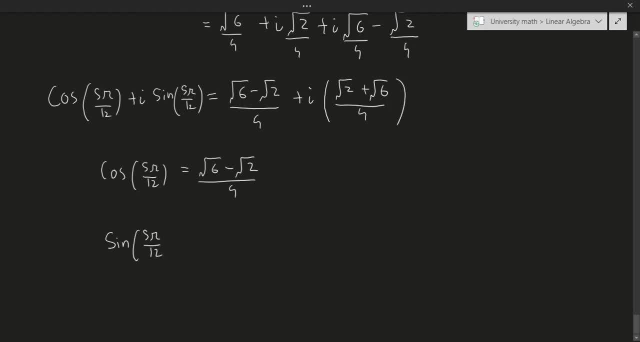 we're going to get sine of 5 pi over 12. right, there is equal to root 2 plus root 6 over 4.. Or, if you want to make this very consistent with the cosine, this is going to be equal to root 6.